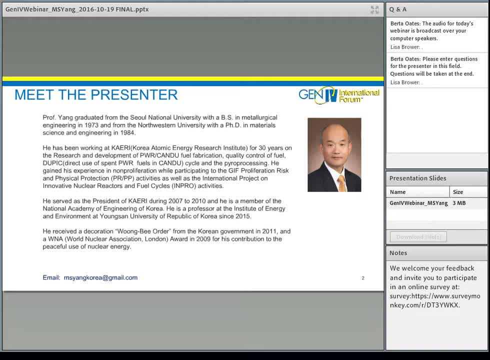 Award in 2009 for his contribution to the peaceful use of nuclear energy. Without any delay, I give you the floor. Professor Yang, I really thank you for volunteering to give this GIF webinar and I'm ready to listen to you. Thank you, Professor Yang. 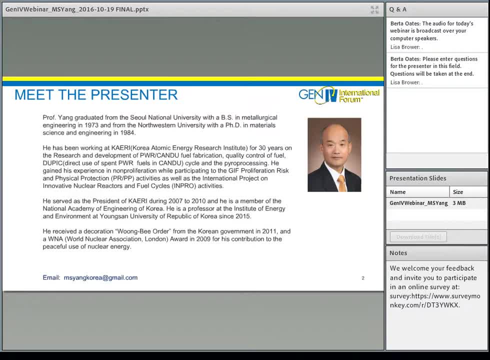 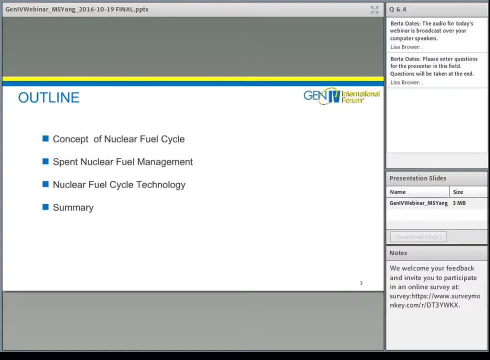 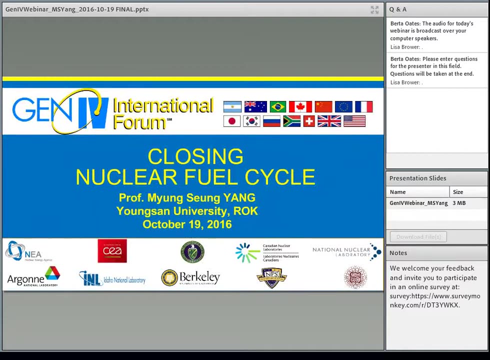 Okay, Thank you, Patricia, for the nice introduction. Hello everyone, I'm Myung-seung Yang and it is my great pleasure to have an opportunity to participate in this webinar. The topic I'm going to talk about today is Closing Nuclear Fuel Cycle, Closing the nuclear 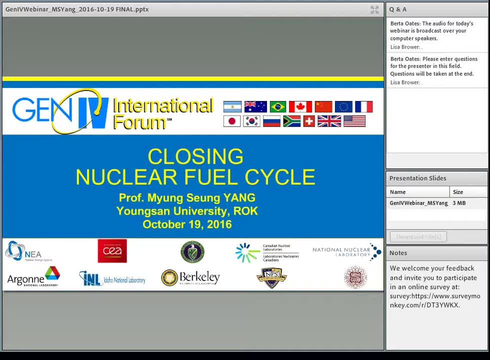 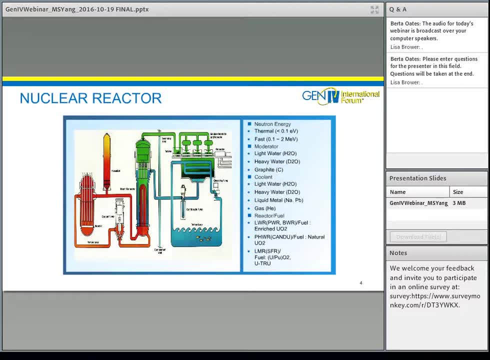 you, Thank you, Thank you, Thank you again. is less than 0.1 electron volt, then there is a thermal reactor and if it is using high energy, fast neutron, or then it is called fast reactor. Also, the reactor can be classified by what kind? 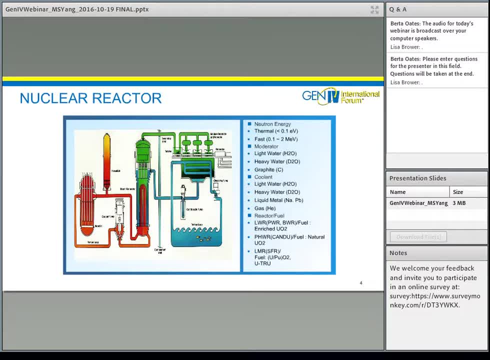 of moderator is used. If it is using normal water, then it is called light water reactor, like PWR and February, and it is using heavy water reactor, then it is called heavy water reactor. it's like a candle reactor, and if it is using graphite, then it is called graphite reactor. 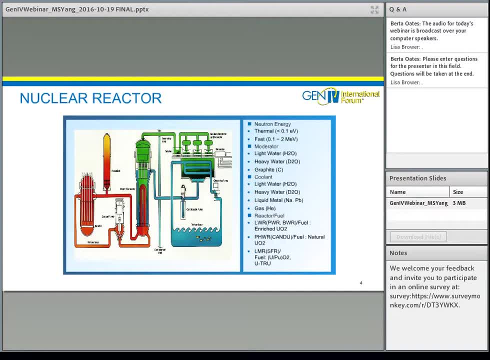 also it can be classified by the coolant. If it is using light water, then it is the light water reactor. if it is using heavy water, then it is heavy water reactor, and if it is using infrared deeper water faster, then it is called rapid-fold-collision water. 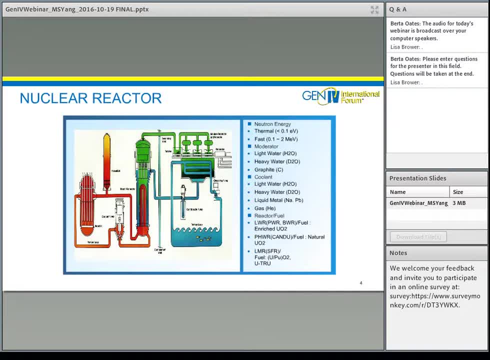 If it is using liquid sodium or lead, then it is called a liquid metal reactor And if it is using helium gas, then it is called a gas-cooled reactor And, depending on what kind of moderator and coolant are used, the type of nuclear fuel. 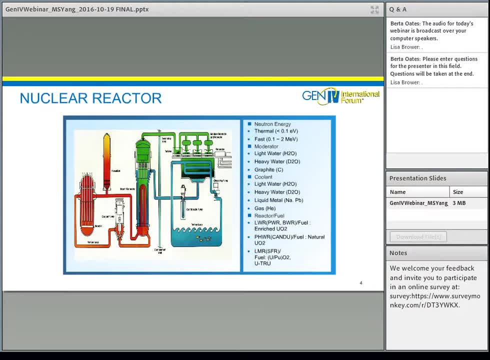 is determined. For example, for the light water reactor, the fuels are made of enriched uranium oxide. The content of uranium-235 in the fuel is about 5%. And for the pressurized heavy water reactor, like a canned reactor, the fuels are made 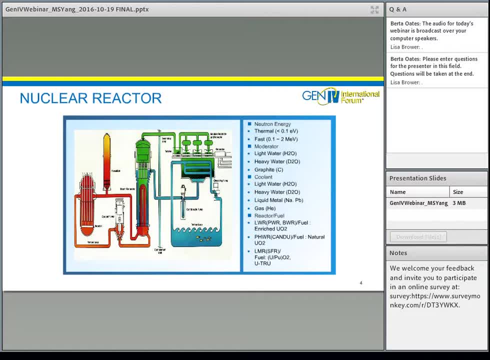 of natural uranium oxide. That means the content of uranium-235 is just 0.7%. And in case of liquid metal reactor, like a sodium-cooled fast reactor, the fuel can be made of hydrogen-235.. Or mixed oxide uranium and plutonium, which is called VOX fuel. 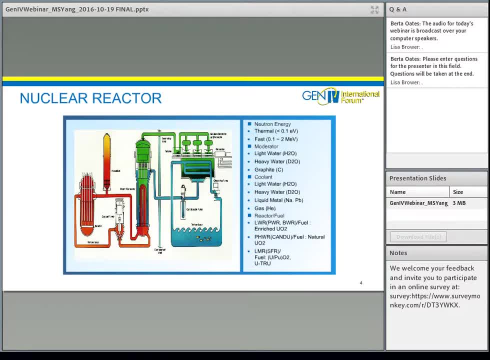 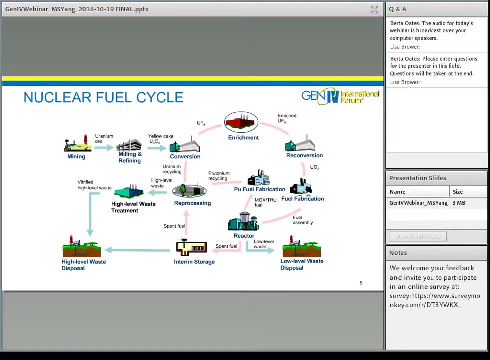 And, moreover, the fuel for SFR also can be made of metallic form, which is made of metallic alloy of uranium, plutonium and other transuranic elements, And this slide shows the concept of nuclear fuel cycle. In this slide, the nuclear fuel cycle is based on the concept of nuclear fuel cycle. 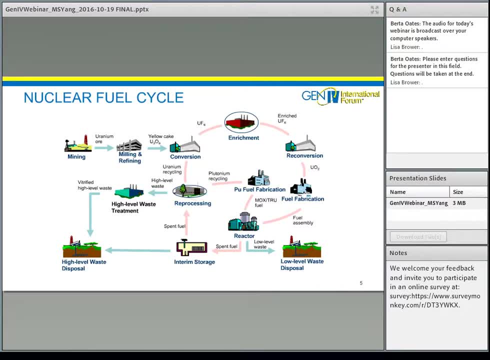 In this slide the nuclear fuel cycle is based on the concept of nuclear fuel cycle. The fuel cycle for PWR is shown as an example. The fuel cycle starts from the uranium mining And after the uranium ores are mined, the impurities are removed at the milling and 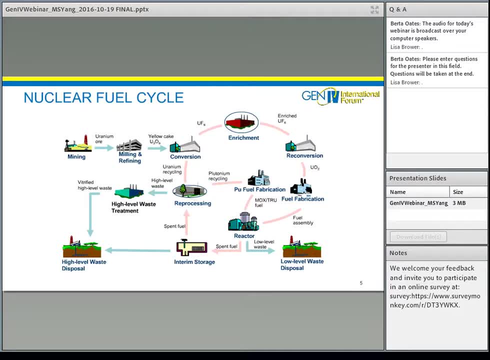 refining process, And then the pure uranium nitrate, called yellow cake, and the uranium oxides are supplied to the combustion plant, And at the combustion process the uranium oxides are depleted. And the uranium oxides are depleted And then the pure uranium nitrate is used in the combustion plant. 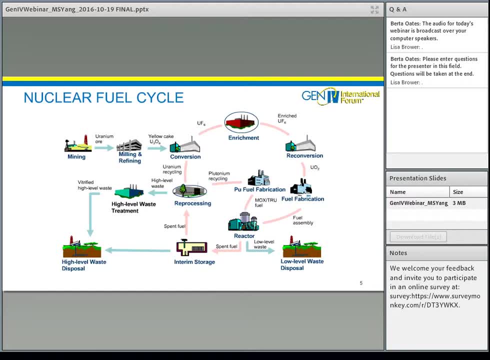 is converted to the uranium fluoride form. then at enrichment stage the uranium fluoride is changed to the gaseous form by heating. then by using this uranium fluoride gas, the isotopic content of uranium-235 can be increased up to 5% to be used for the nuclear fuel. The 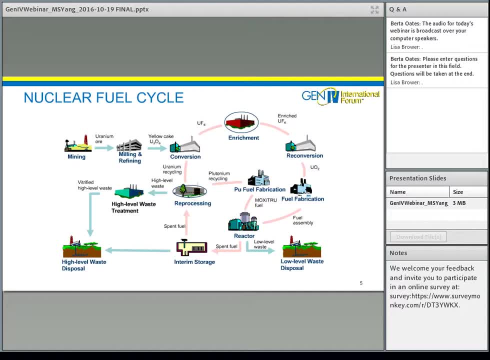 enriched uranium fluoride is deconverted to enriched uranium oxide at the decombustion plant. then the enriched uranium oxide is fabricated to the nuclear fuel assembly by using powder metallurgy technique with zirconium klaggin tube and with other structural parts. then nuclear fuel assembly are loaded to the nuclear reactor. 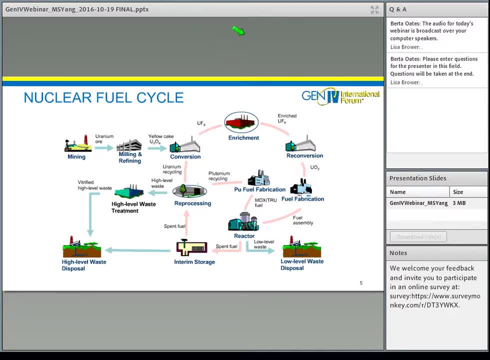 and the bond at the reactor. four and three years to generate electricity, And the process steps from the uranium mining to the fuel fabrication before loading to the nuclear reactor is called front-end fuel cycle And after three years of burning in the reactor the fuels are discharged from the reactor. 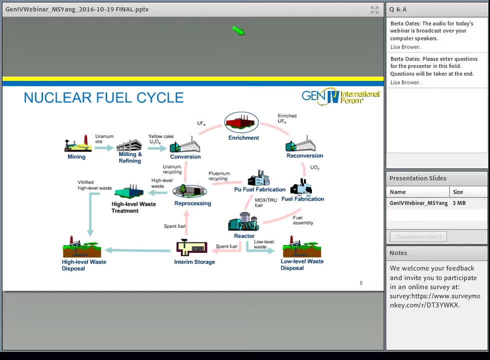 as a spent fuel. Nowadays, frequently it's called as a used fuel, And the process steps from the discharge of the fuel from the reactor and the following processes are called as the back-end fuel cycle. And in the back-end fuel cycle there are various ways to treat the spent fuel. 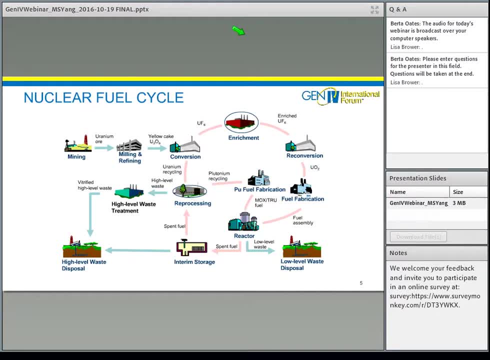 The simplest one is the spent fuel is stored at the interim storage facility for a period of time. Then the spent fuel is buried under the ground at the high-level waste disposal site, And this type of fuel cycle is called once-through fuel cycle or open fuel cycle. 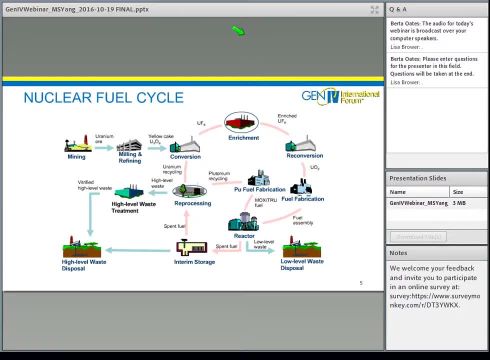 And the other way is the spent fuel from the interim storage is moved to the reprocessing facility, And at reprocessing the remained uranium and the newly produced fuel are stored in the heating facility. In the back-end fuel cycle the newly produced plutoniums are recovered from the spent fuel. 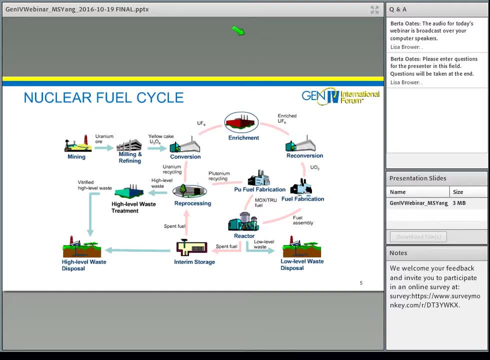 And then the plutonium is fabricated as the plutonium-bearing mixed oxide fuel or the TRD fuel, which will be re-burned at the reactor. And after the plutonium-bearing fuel is re-burned at the reactor, the spent mox or TRD fuel. 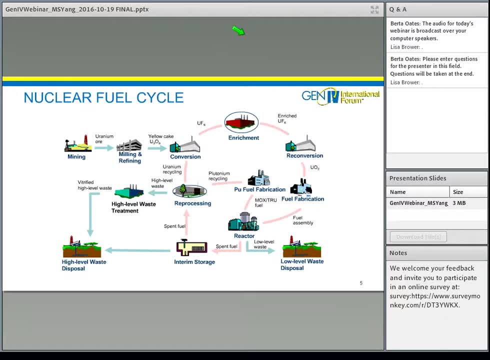 will be again reprocessed to remove the impurities. So now theес, there's a lot of waste in the reactor. These are all of the chemical waste- and to recover the uranium and plutonium and which will be again refabricated as a fuel. So, theoretically, this type of 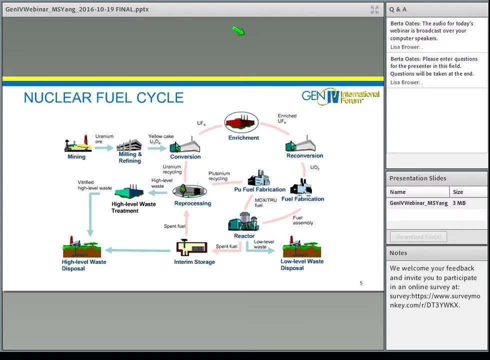 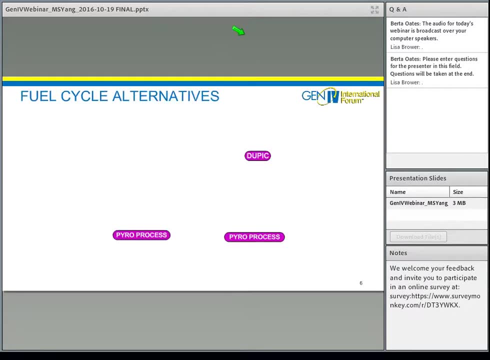 recycling is possible for the several times. So this type of fuel cycle is closed fuel cycle And this slide shows schematically several examples of the possible fuel cycle alternatives. Regarding back-end fuel cycles, theoretically many fuel cycle alternatives are possible. They say more than 60 fuel cycle alternatives are possible, but 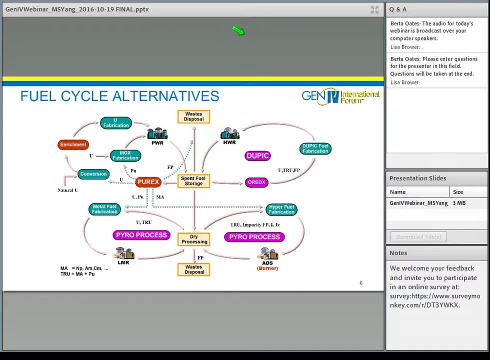 there are two main routes, that is, the one is dry process root and the other one is the wet root, and first one is spent fuel will be treated by the wet process, or called the purex process, to recover the remained uranium and plutonium. then the recovered plutonium is fabricated as a mocked fuel and also for the 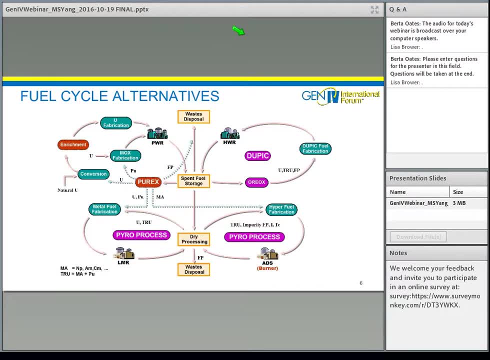 recovered uranium, it will be converted to the fluoride form and it needs to be to be used as the uranium fuel for the pwr reactor. and the second one is the spent fuel will be treated by the dry process called the pyro processing to retrieve the remained uranium and plutonium. 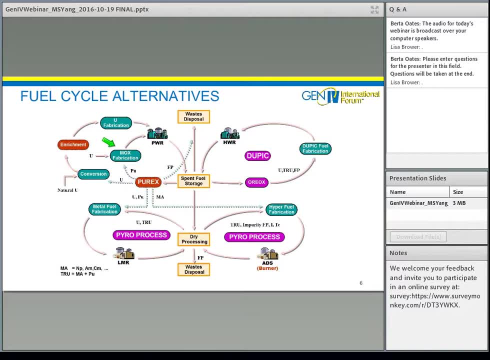 with other trial materials and then the uranium and the trial materials will be fabricated as a fuel for the fast reactor like a sodium cooled fast reactor. and the other possible way is a pwr fuel is directly refabricated for the fuel of heavy water reactor like a candle or as the content of the fissile material in the spent pwr fuel is large. 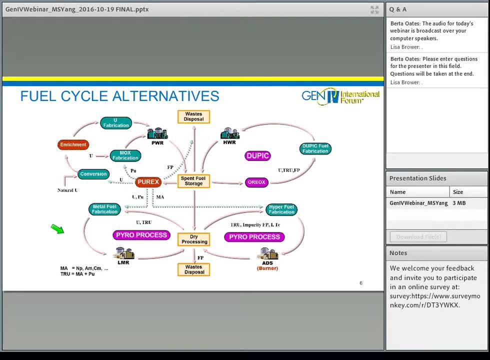 enough to be used in candleware reactor whose fuel is made of natural uranium, and this process is called the root process. and the other option is the spent fuel is treated by dry process to recover the trans-uranium material with fission products like iodine and technetium, and then the material is fabricated. 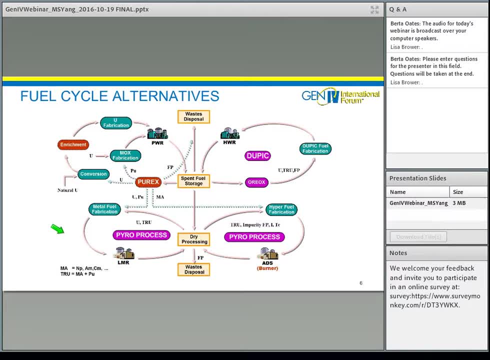 as a target for the accelerator accelerator driven system, and at the accelerator driven system the long-lived fission product will be transmitted to the short-lived short-lived element. so this will be beneficial for the management of HEGADOS long-lived fission program. so this is called HYPER system. HYPER stands for the hybrid power extraction reactor. 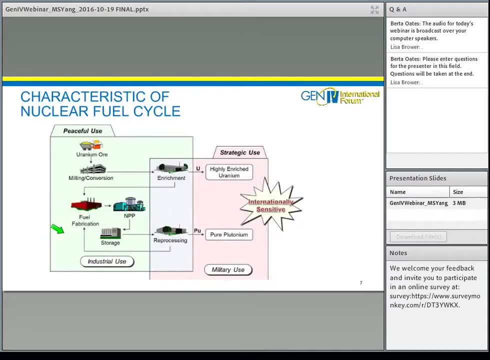 so when we are dealing with nucleus of the nuclear system, we are also dealing with nuclear power extraction fuel cycle. one important issue is nuclear non-proliferation. So for the enrichment process in the front-end fuel cycle, since the highly enriched uranium can be used for the nuclear weapon material, the enrichment process is the internationally 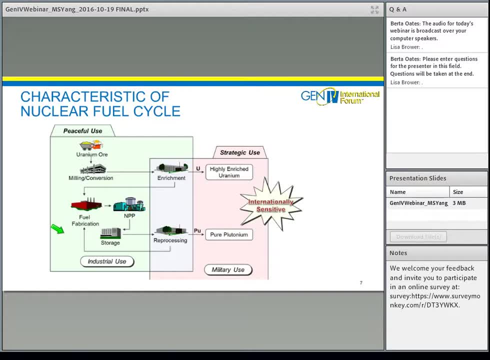 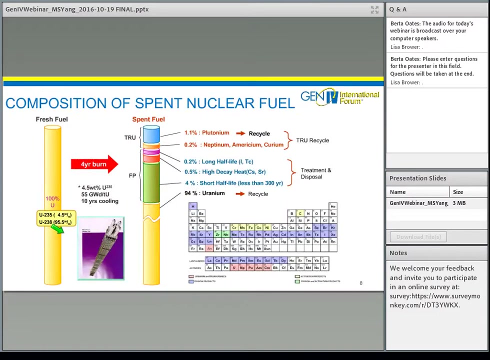 sensitive area And for the reprocessing steps in the back-end fuel cycle, since the pure plutonium can be used for the nuclear weapon material. so the reprocessing process especially, which can produce the pure plutonium, is also an internationally sensitive area. 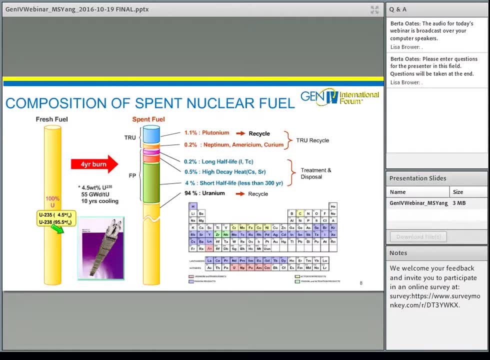 And this slide shows a typical example of the composition of the spent fuel. Surely, the spent fuel has various compositions. The spent fuel is based on the initial enrichment level and the burnout history at the reactor- In case of 4.5% U-235 enriched fuel which is burned up to 55 gigawatts. then the composition. 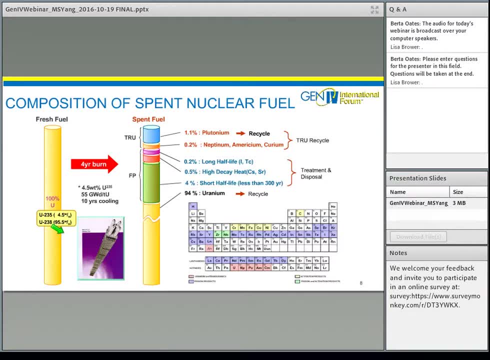 of spent fuel roughly looks like this: The fresh nuclear fuel is made of 100% pure uranium, But in the spent fuel the spent fuel is made of 100% pure uranium, So the spent fuel is made of 100% pure uranium. 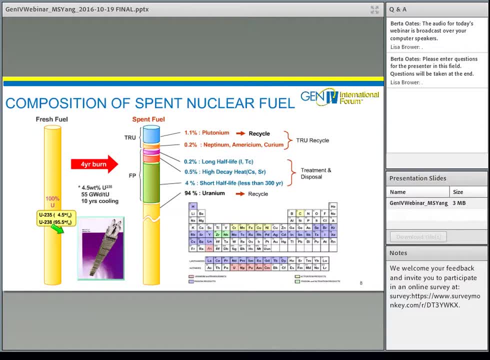 The 94% of spent fuel is composed of the remained uranium, So it means only about 6% of uranium is burned in the reactor, And during the burning the uranium is converted to the plutonium And the amount of plutonium is about 1%. 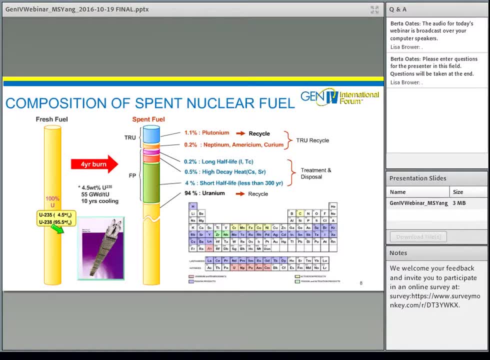 And 0.2% of spent fuel is minor ethylene. And 0.2% of spent fuel is minor actinide elements, such as neptunium, imidacium, cubium and so on. And the plutonium and the minor actinide elements are called TRU elements. that means transuranic. 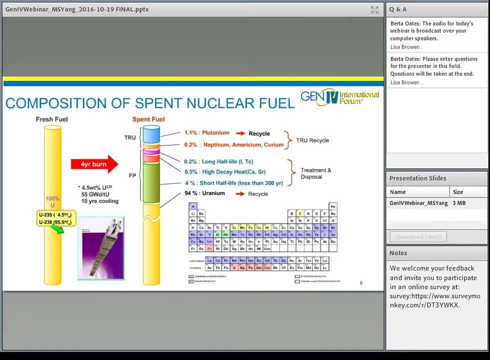 elements And during the fission. various fission products are produced, And among them several elements need special attention. Iodine and technetium have a long half-life. They are long-lived fission products which indeed have a longer period of special care. 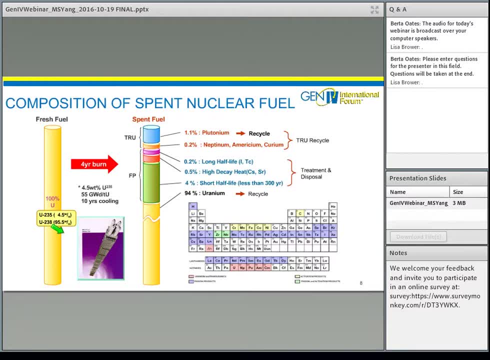 for the permanent disposal, And the amount of these long-lived fission products are about 0.2%, And some fission products, like cesium and strontium, have a high decay heat, which also means that they need special care for the permanent disposal. 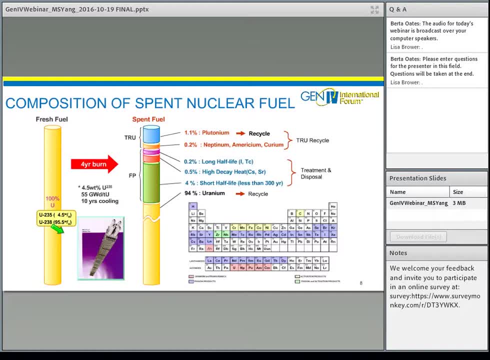 And the amount of high decay heat elements are about 0.5%. And the remaining fission product has a short half-life- less than 300 years- And its amount is about 4%. So therefore, for the best management of spent fuel, we need to close the spent we need. 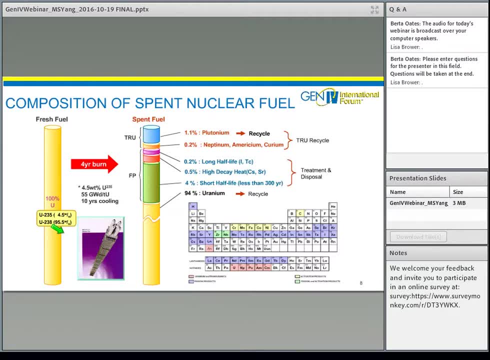 to close the fuel cycle. That means reusing the remaining fissile material in the spent fuel And that means the 94% of the remaining uranium and the 1.3% of TRU material will be recovered and recycled in the reactor. 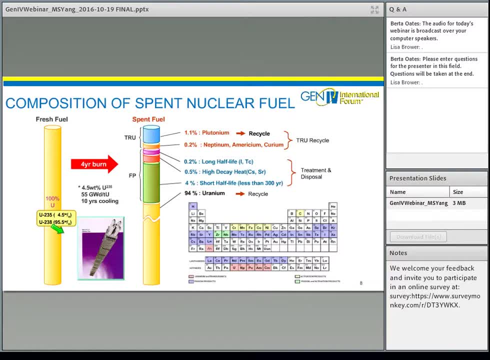 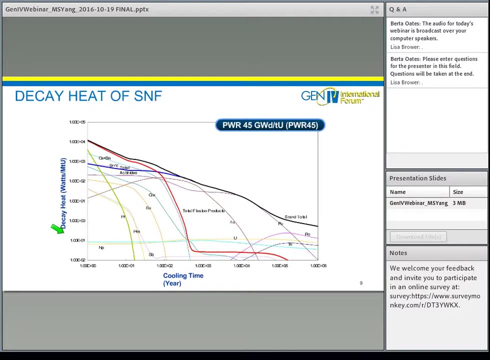 And about 5% of fission products will be separated and specially treated and disposed of permanently. And that's the end of this presentation, Thank you. And this slide shows the amount of decay heat generated, which decreased as time passed by. When nuclear fuel is irradiated in the reactor, some elements become unstable. 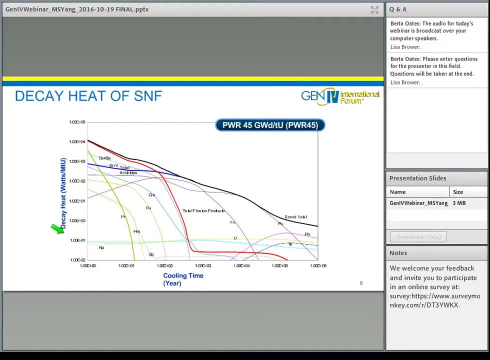 So they tend to be changed to the stable state by emitting heat, And we call this the decadal heat. The amount of decay heat and its change over time is a very important factor for the permanent disposal of spent fuel. The decay heat is the characteristic of spent fuel. 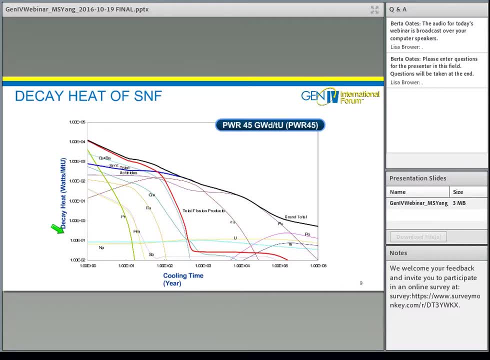 That is, even though nuclear fuel is discharged from the reactor, the spent fuel generates decay heat, So spent fuel should be cooled down for a period of time. For example, in case of uranium, the amount of decay heat is 0.1 watts. 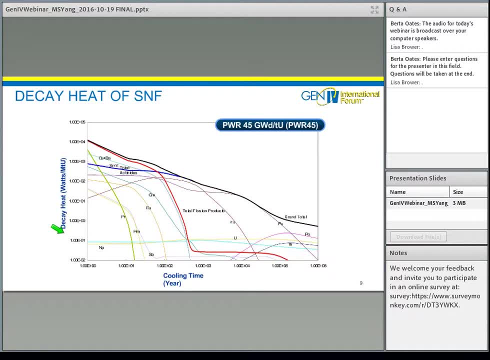 It's quite small, but it does not change much with time. In case of Plastidium the decay heat is about 5,000 watts and it's quite large, but it is decayed. It's decreasing quite fast, so it is almost zero in 20 years. 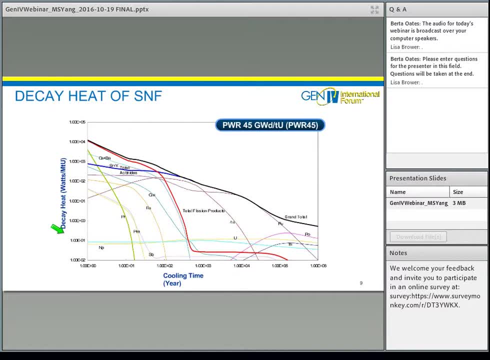 And in case of Plutonium the decay heat is around 200 watts and it is relatively large and it lasts a very, very long time. So it needs almost 1 million years to be cooled down Collectively. the change of decay heat from spent fuel to spent fuel is very significant. 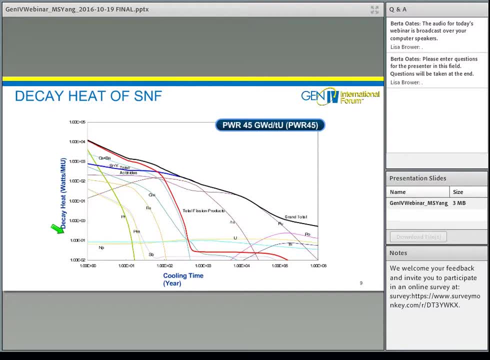 The decay heat from the old fission products are shown in this red curve. So it shows that the decay heat from the fission products will be cooled down in about 300 years, And the change of decay heat from old actinides, including Plutonium and Ameritium, et cetera. 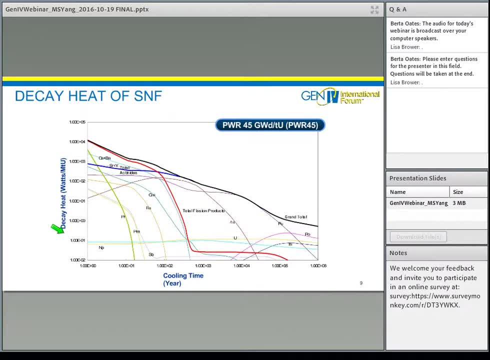 are shown in this blue curve. The initial decay heat is large, about 1,000 watts, And it lasts about 1 million years to be cooled down. So the change of the grand total value of decay heat are shown in the black curve. 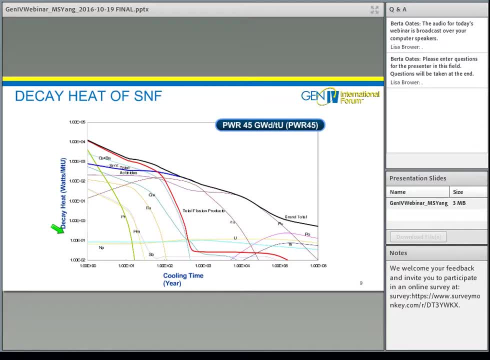 The initial value is large and it also lasts very, very long, mainly because of the TIL element. So, therefore, this fact is the reason why we need to reprocess the spent fuel. That is, the actinide elements are separated from the spent fuel and they will be re-burned. 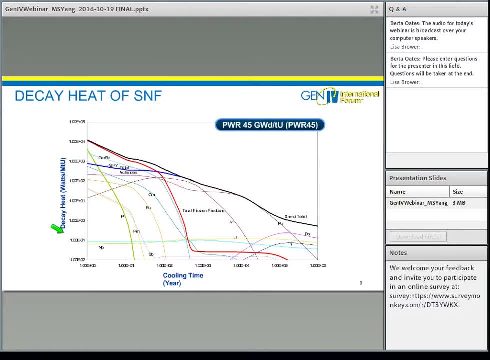 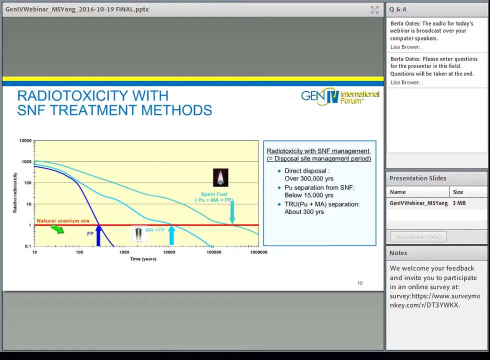 at the fast reactor And if the TIL elements are removed from the spent fuel, then it will only need about 300 years to cool down the decay heat. And this slide shows the comparison of the radio toxicity For the spent fuel which contains the Plutonium, minor actinide and all the fission products. 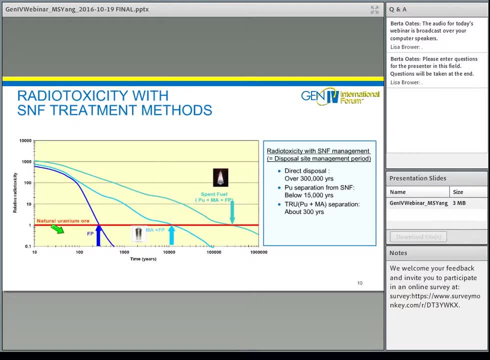 the value of radio toxicity is about 1,000 times larger than that of natural uranium And it takes about 300,000 years to decrease to that of natural uranium. So that's the difference, Thank you, And for the materials which contains minor actinide and fission products without Plutonium. 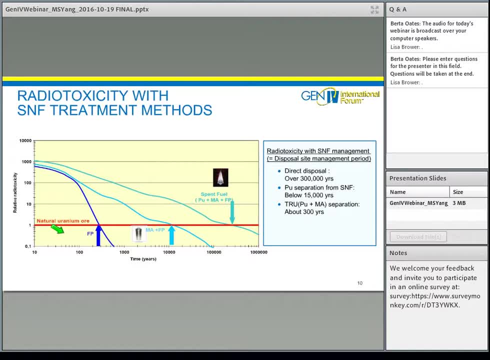 it takes about 15,000 years to become natural uranium level, And for the materials which contains only fission products, without Plutonium and the minor actinide, it will take about 300 years. So this time to decrease the radio toxicity to the natural level is the time period for. 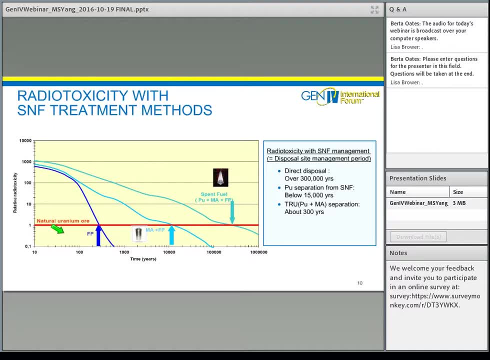 which we need to manage the permanent waste disposal site. So if the spent fuel is not treated at all and directly disposed, then waste disposal sites are needed to be managed over 300,000 years. But if all the TIL materials are not treated at all and directly disposed, then the waste 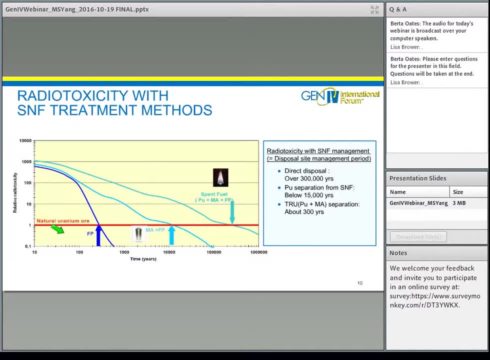 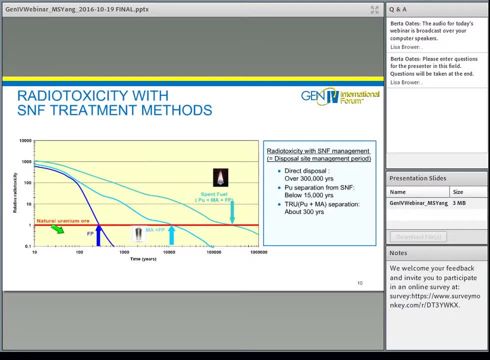 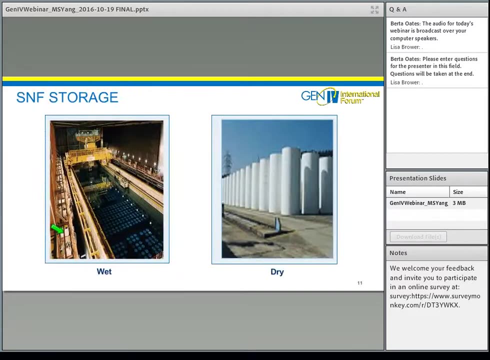 And this is why we are developing the advanced fuel cycle to remove the TRU element and reuse them by burning a fast reactor. So that is to close the fuel cycle. Regarding the internal storage of the spent fuel: when the spent fuels are discharged from the reactor they are normally stored under the water for about 10 years to cool. 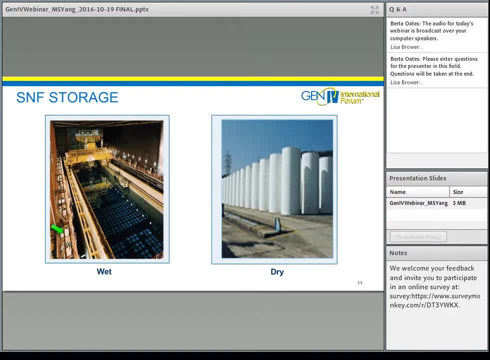 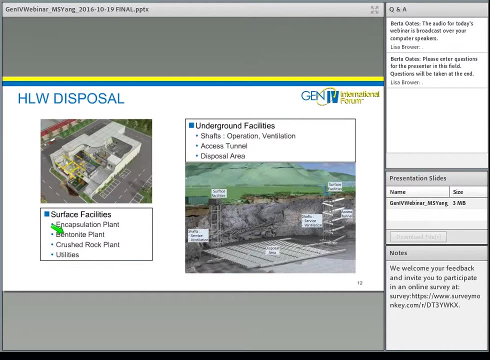 down the decay heat. Then, after 10 years of wet storage, they can be moved to the dry storage canister to store them more economically. Eventually, this is the end of the story. Finally, the spent fuel and the high-level waste will be moved to the repository for. 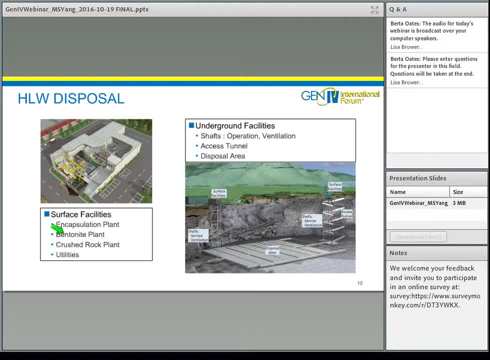 the permanent disposal, And this slide shows the typical example of permanent disposal sites. On the surface there are encapsulations and the bentonite plant to seal the radioactive waste and the other service facilities, And under the ground there are boreholes. 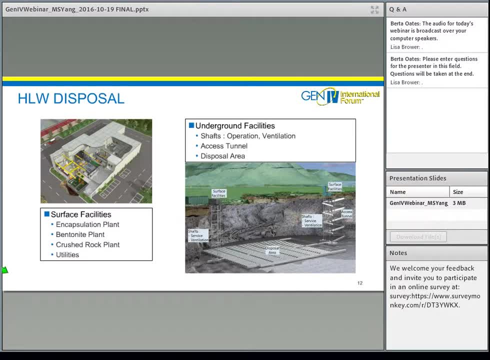 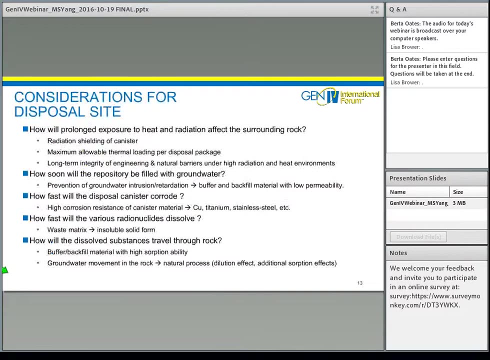 And under the ground there are boreholes, There are vertical shafts for service activity and ventilation And there are horizontal tunnels to store the encapsulated waste safely for long periods of time. When we select the permanent disposal site like this, there are some special considerations. 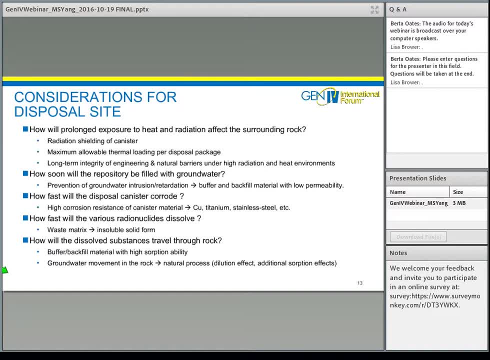 needed. So they are. how will the waste be stored? How will the prolonged exposure to heat and the radiation from the waste affect the surrounding rock? So that is, the long-term integrity of the engineering and the natural barrier on the high radiation and the heat environment is important. 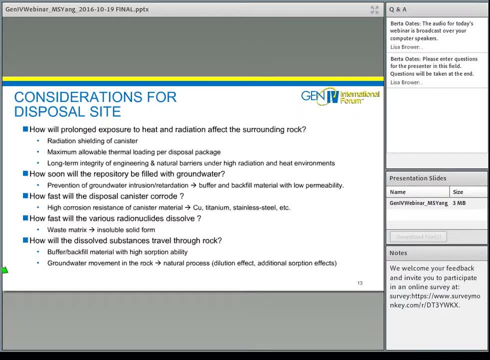 So we should consider radiation shielding of the canister and the maximum allowable thermal loading of the canister. And the second point is: how soon will the repository be filled with groundwater? That is the prevent of groundwater intrusion. So this requires the selection of a buffer and the backfill material with low permeability. 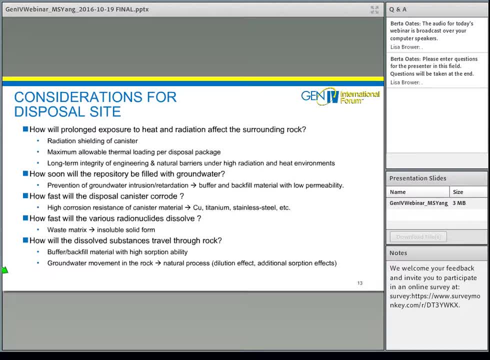 And the third thing is: how fast will the disposal canister corrode? The disposal canister must be successfully filled, because the disposal canister is likely to corrode. And'll follow the same principle in the next slide. So that is our analysis. 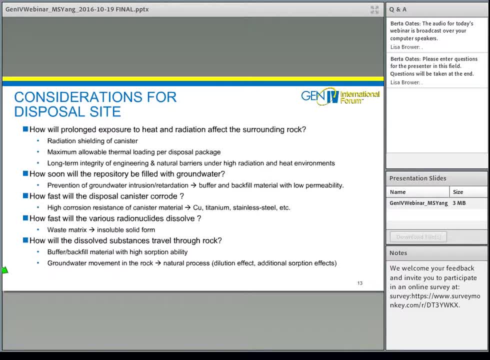 Now the third point is: how quickly will the disposal canister corrode? So usually, when the disposal is filled with water, the capacity of the disposal canister is very limited. So this requires that the canister is made of high corrosion resistant material like 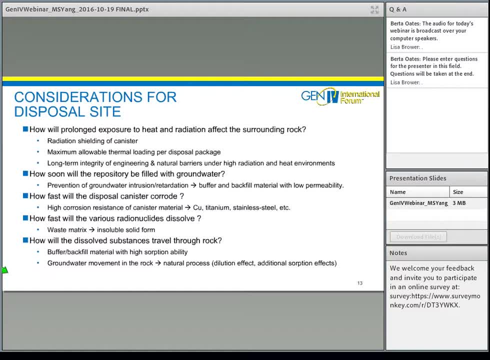 copper, titanium and stainless steel, etc. And the fourth point is: how fast will the various radionuclides dissolve And how will the dissolved substance travel through the rock? So the groundwater movement in the rock is an important factor. So, considering the long-term integrity and the safety of the disposal, it is not easy. 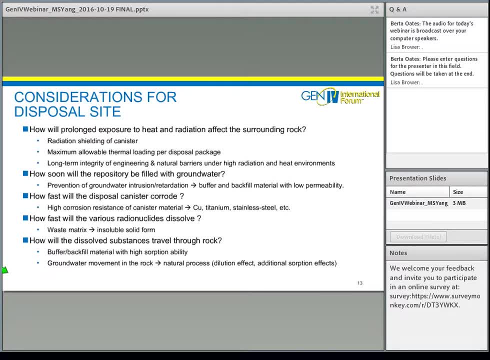 to select the proper waste disposal site in terms of engineering viewpoint. Moreover, it is also not easy to get the public consent and acceptance. So currently there is no public consent And many countries, including South Korea, have such a challenge to select the waste. 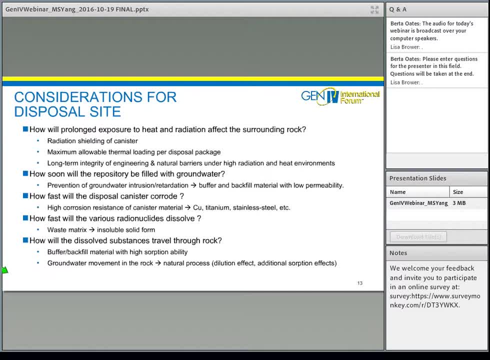 disposal site. So this is another reason why we need to develop the advanced fuel cycle technology to close the nuclear fuel cycle in purpose of to reduce the amount of radioactive waste and to reduce the necessary area for the permanent disposal of the spent fuel And to decrease the time period needed to manage the final disposal sites. 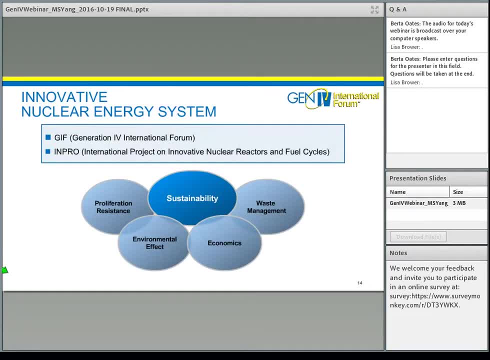 1. GIF and IAEA In the fall of 2000,, there are some international efforts to develop innovative nuclear energy systems. The main activities are led by GIF and IAEA. The objective of this effort was to organize two nuclear facilities. efforts for innovative nuclear system are to improve the sustainability and for the 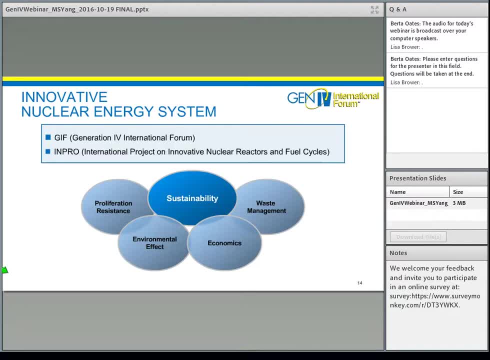 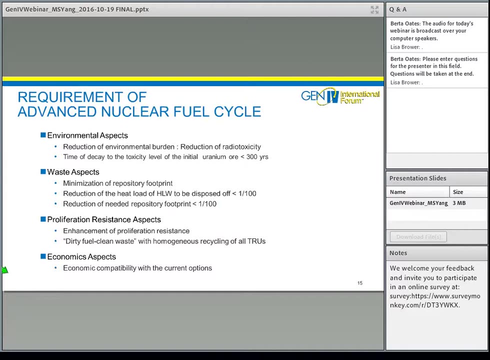 optimal waste management and the environmental effect and improving the economy and also enhancing the proliferation resistance. And this slide shows the basic requirements of the advanced fuel cycle For the environmental aspect: we easily reduce the environmental burden by reducing the radio toxicity of spent fuel. 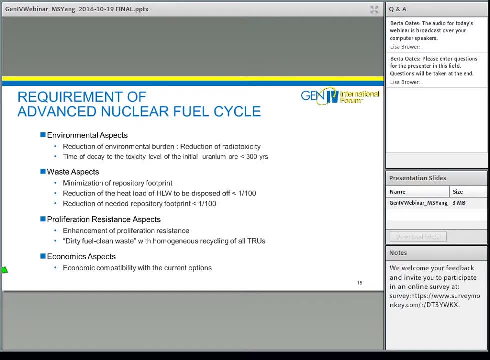 So the target is the decay time of spent fuel to the toxicity level to the natural uranium should be less than 300 years And for the waste It will minimize the required repository footprint. So that is, by reducing the sheet load of waste by 100, the necessary repository footprint. 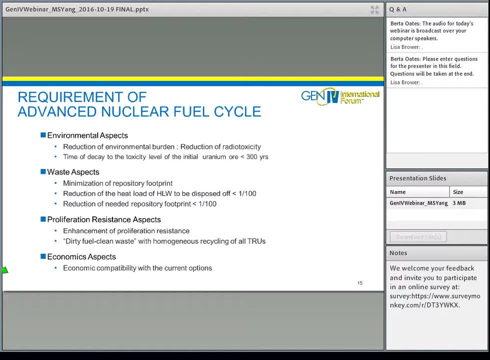 also can be reduced by 100.. And for the proliferation risk aspect, the proliferation resistance can be enhanced by recycling all the material Together, based on the concept of so-called dirty fuel, clean waste. And for the economical aspect, the new technology should be economically compatible with the 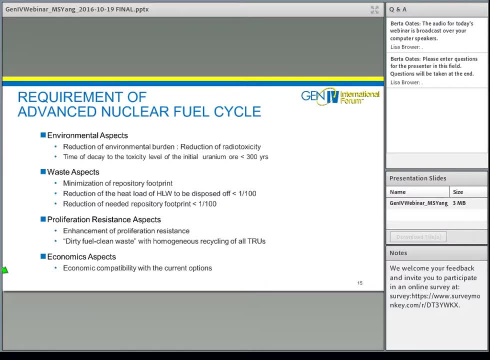 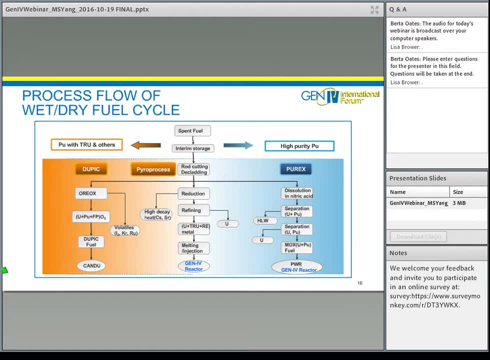 current technical option, Even though a lot of technology alternatives are proposed For the treatment of spent fuel. it can be classified by two methods. They are wet processing routes, like Purex, and dry processing routes, like pyroprocessing, And I'm going to explain this process in more detail at the following slide. 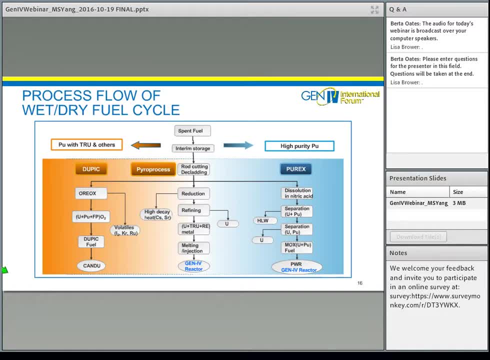 The product from the Purex process can be used for the PWR and the Gen IV reactor as a maximum, And the product from the pyroprocessing can be used for the fuel of the Gen IV reactor as a metallic fuel, And one of the interesting concepts is DUPIT. 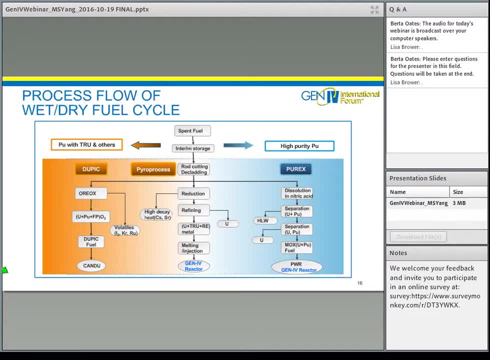 So where the spent PWR fuel will be directly refabricated as a fuel for the canned type reactor. So this is a typical example of the concept so-called the dirty fuel. And this is a typical example of the concept so-called the dirty fuel. 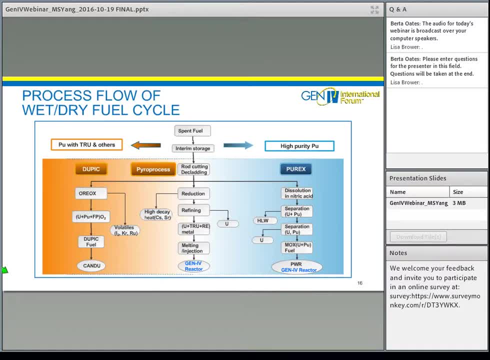 And this is the clean waste. So in fact we tried to make a nuclear fuel with high purity material in order to attain high burnup and therefore easy of the fuel management. But this produce radioactive waste. So recently we tried to make a fuel with the uranium and the element, and they will be. 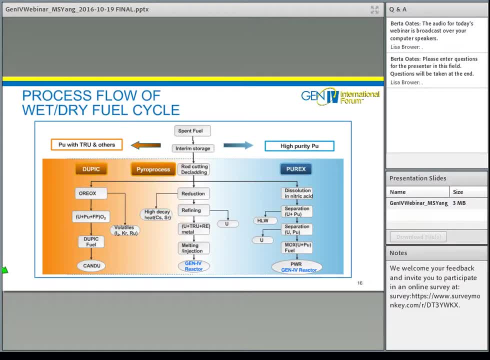 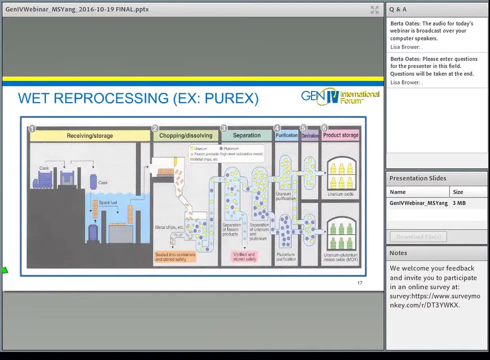 reborn at the reactor. So in this example this is a nuclear fuel. So in this way we can make it easy to manage the clean radioactive waste. So this slide shows the process flows of each reusing process And this slide shows the overall process flow of ready processing like a purex process. 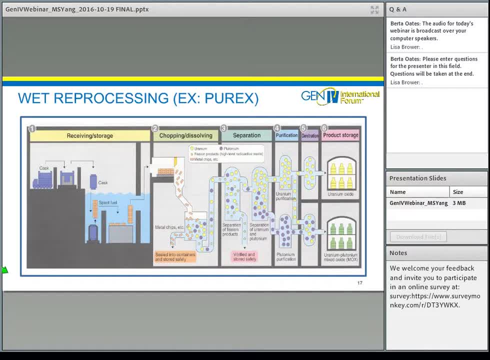 So it's composed of six areas. So first is receiving the spent fuel casks and they will be stored under the water, And second is disassembling, capping and the dissolving area. So here the fuel assembly is capped to the small piece and they will be dissolved in the nitric acid. 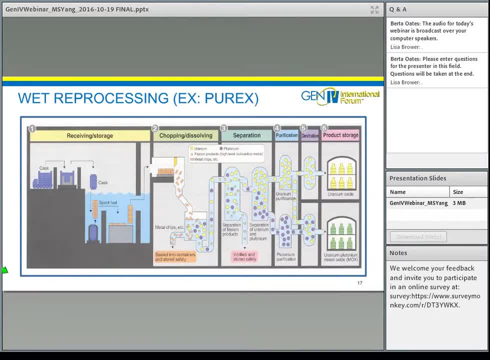 And in this process uranium, copper and silicon are dissolved. Plutonium and some fission products are dissolved in the nitric acid, but the metallic parts, like cladding tubes, are not dissolved. So this kind of solid metallic part can be separated from nitric acid fuel solution, And those stages are called head-end. 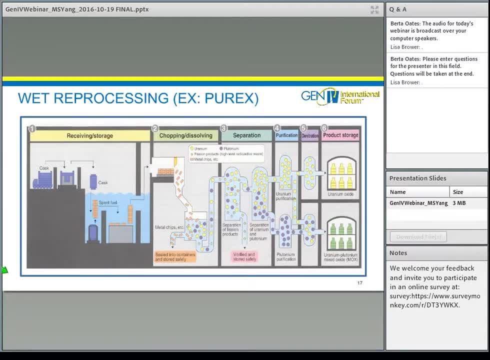 process. And third area is the separation area. So here it is to separate the uranium and the plutonium solution from the fission product by using solvent extraction, Then by using the uranium and plutonium mixtures which are free from fission product. 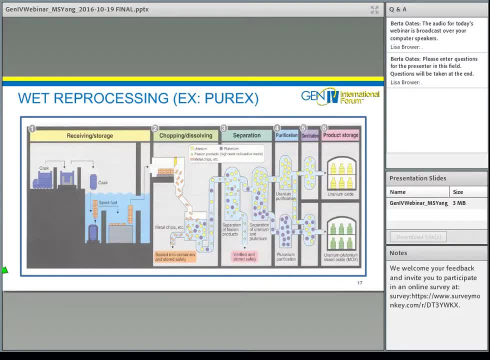 plutonium can again be separated from uranium by solvent extraction. And the fourth area is the purification area, So it is to purify a separated solution from uranium and plutonium from remaining impurity by using solvent extraction. And fifth area is denitration area, So it is to denitrate the uranium and plutonium nitrate to 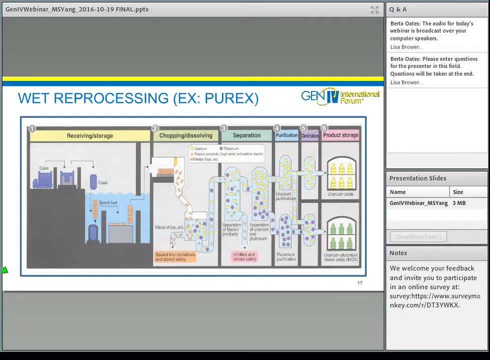 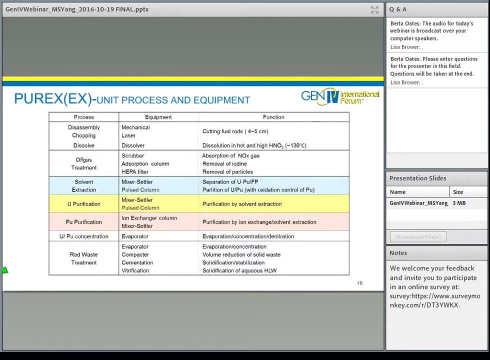 produce pure uranium and plutonium material. Then uranium and plutonium is converted to oxides for storage of the main equipment and its function in the purest process. for the disassembly and the charging of the fuel, mechanical and the laser method can be used. 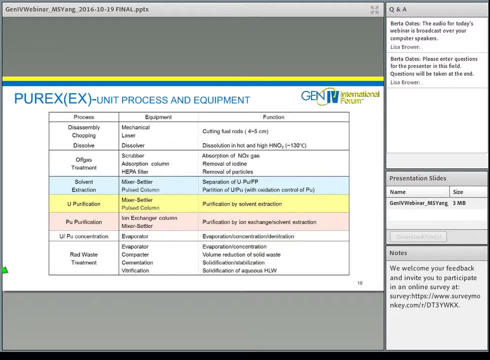 And dissolving is to dissolve the fuel material in nitric acid, and here the fuel material can be separated from the structural part, And during this process radioactive gases will be released from the fuel. So this off-gas treatment by adsorption columns and HEPA filter is also an important area. 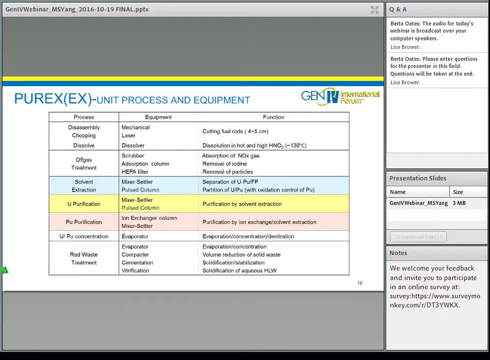 And the uranium-plutonium extraction. purification can be performed by solvent extraction methods by using equipment like a mixer settler and the first column. Then pure uranium and plutonium material can be produced by the denitration using evaporators And along with these processes, the radioactive process. waste treatment is also very important. 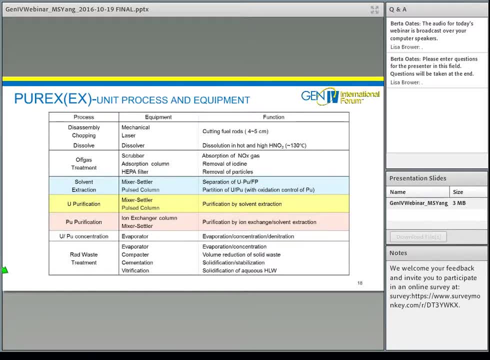 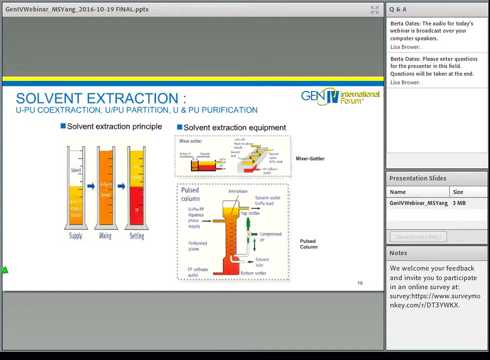 So the waste is the volume reduced by evaporator and the compactor, and then it will be solidified by the cementation and the vitrification. So this is the end of the presentation, Thank you. So this slides shows the basic concept of solvent extraction, which is commonly used. 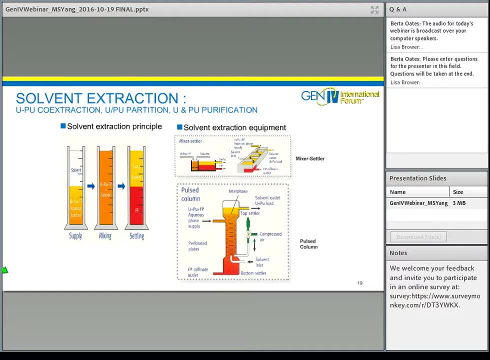 in the ordinary chemical plant. So that is solvent and the fuel solution with the fission product will be mixed together. Then on dissolving fission product will be settled down to the bottom part And the uranium and plutonium which are dissolved in the solvent will be mixed together. 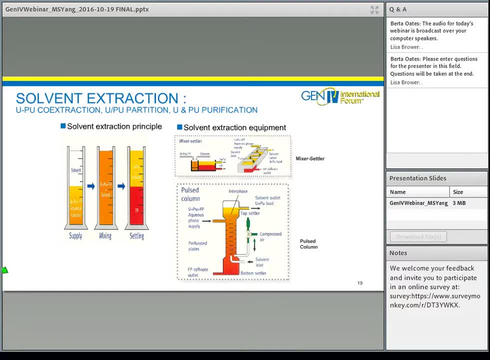 And the thermo and nitrate dissolved in the solvent will be located at the upper part. In this way they can be separated each other. So in this process- the most popular process- equipment used is a mixer settler or first column, And this type of mixer settler can be arranged in series to repeat some mixing and the settling. 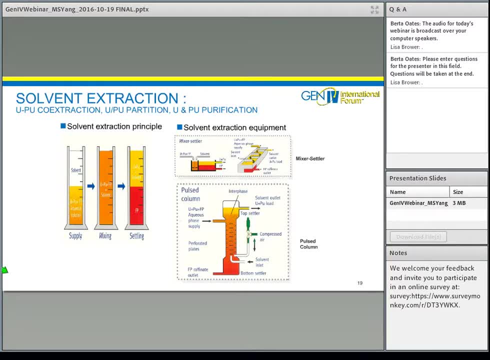 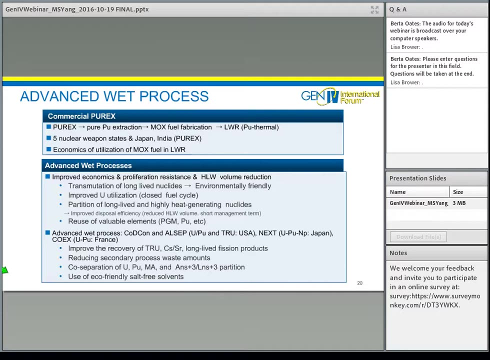 process to achieve higher purity. Thank you, Thank you for your attention. The first column has very similar function regarding the mixing and settling by pulsing. So nowadays, purex process is well developed and commercialized by the five weapon states, Japan and India. 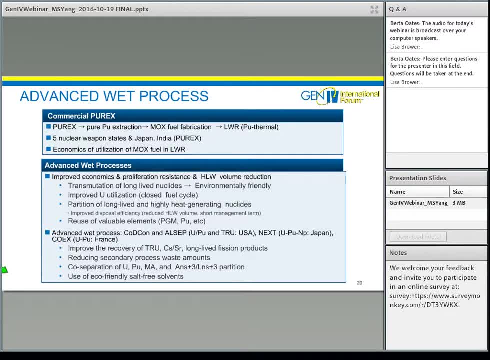 By using purex process, uranium and plutonium oxide mixed fuel, called MOX fuel, can be fabricated and it can be used at the current light water reactor and this is called flue thermal recycling. However, nowadays, more advanced jet reprocessing is under development to improve the economic 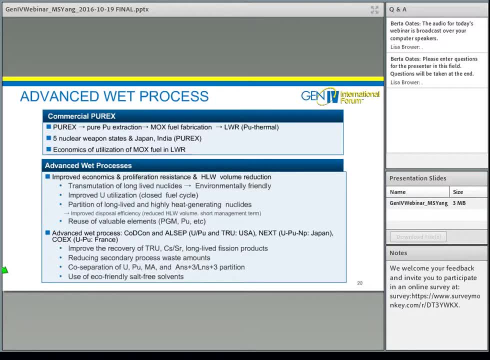 proliferation rate. It has been added to the new capture plant to produce a higher level volume resistance and the volume reduction of the higher level waste. That is, by producing uranium and plutonium with other long-lived nuclides together and by burning them in fast reactors they can be transmitted to the short-lived elements. 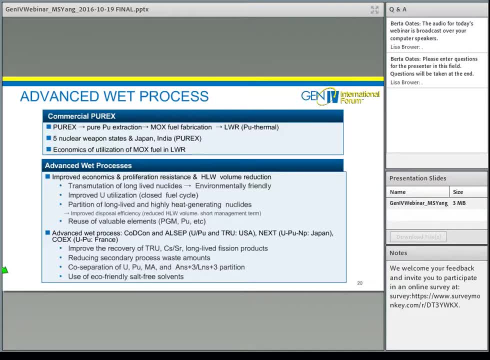 for environmentally friendly recycling, Also by recovering uranium and the self-contained material from nuclear reactors. they can be like plutonium in the spent fuel and burning them. we can improve the uranium utilization by completely closing the nuclear fuel cycle And, moreover, by partitioning the long lived nuclides and highly heat generating elements. 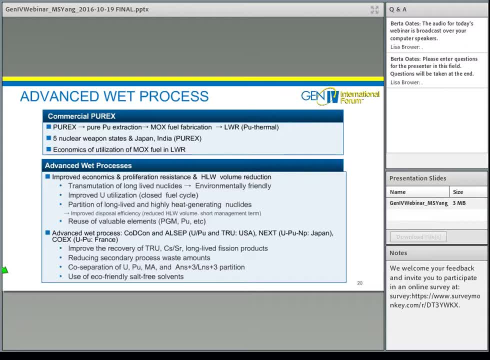 from the waste. we can improve the efficiency of permanent waste disposal by reducing the volume of high level waste and by shortening the management period of permanent disposal time, And several advanced web processes are under development, such as cold contamination and the alkalized and lanthanized separation process. 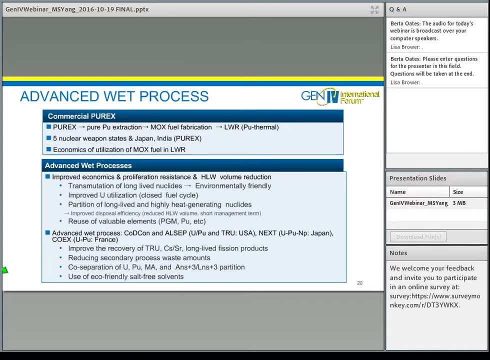 The next process is to separate uranium, plutonium and TRU together in the USA. And the next process development is to separate uranium, plutonium and neptunium in Japan. And the next process development is to separate uranium, plutonium and neptunium in Japan. 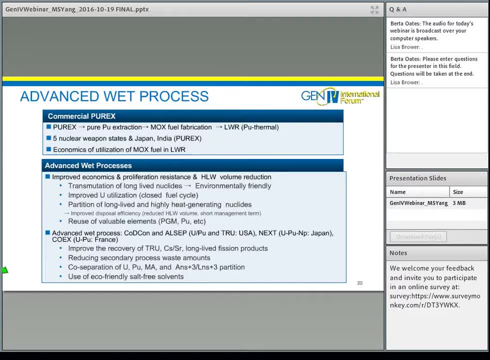 So mainly the objectives of this technology development are To improve the recovery of TRU, cesium tritium, which are high decay heat elements and also long lived fission elements, And to reduce secondary process waste amount And to co-separate uranium, plutonium and lanthanide partition. 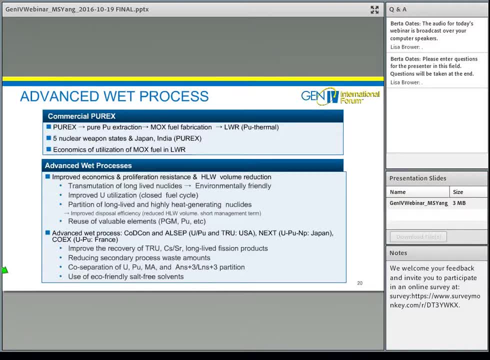 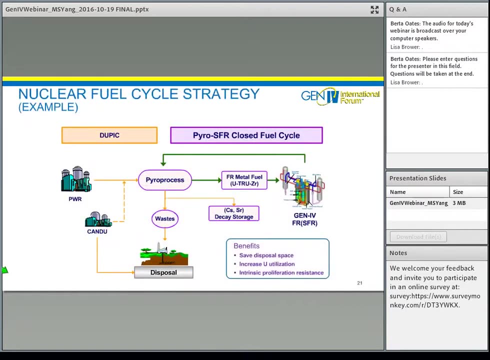 And to use the EcoFrame. And to use the EcoFrame- The products that we grow in Japan, And to be able to digest, recycle, Reuse And to use these products to produce renewable energy 힘 during water quality, even in. 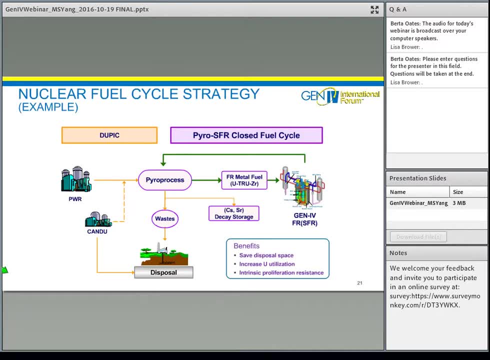 the climate. So in 2012, we conducted a specific in the United States: the interest teaspoon experiment that we conducted in bay lands 10 years ago, Eight years ago. the fast reactor, So spent PWR fuel, can be directly fabricated as a dupic fuel to be used. 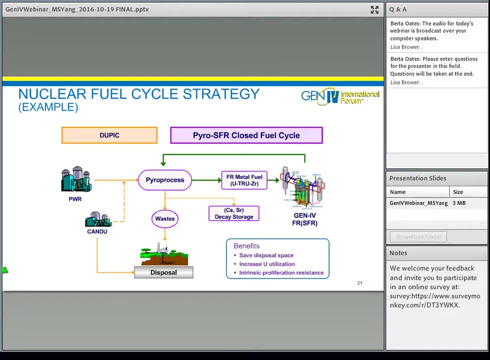 at the canned reactor and also spent PWR can be treated by the dry pyro processing to produce the metallic fuel made of uranium and the child element and the zirconium. Then they will be used as a fuel for the sodium, cold fast reactor and in this way we can save the permanent disposal. 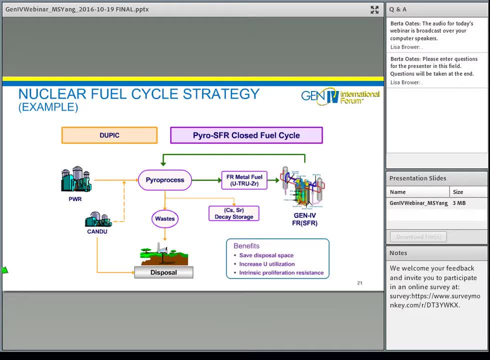 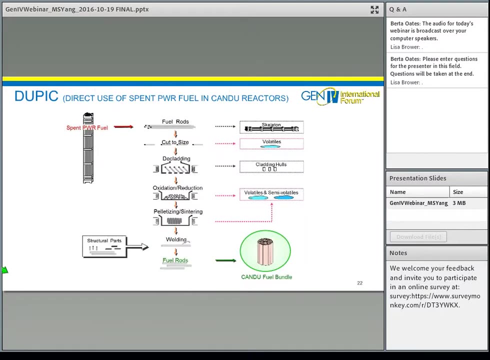 space of the waste and it can improve the uranium utilization. and also this dry process has the intrinsic proliferation resistance. So this slide shows schematically the process flow of the dupic fuel fabrication. So the spent PWR fuel is disassembled and cut to small pieces and 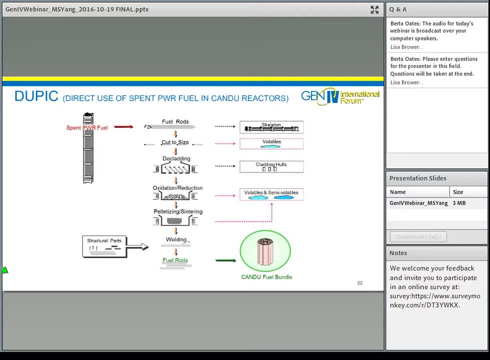 they are declared by mechanical and thermal methods. Then the spent fuel materials are treated by a series of oxidation and reduction to make the fuel powder the soft and the porous and the resin terrible. and once the resin terrible powder is prepared, then the The remaining fabrication processes are the same as the typical fabrications. 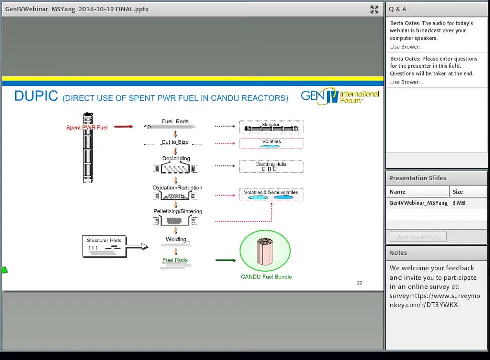 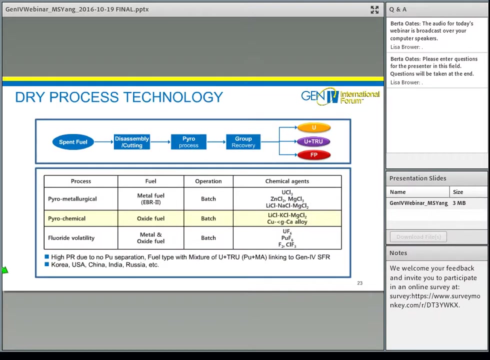 So this concept has been proved at the laboratory scale and the performance was evaluated by the evaluation at the research director in cooperation with South Korea, Canada and the USA. but it has not been commercialized, And this slide shows the characteristics of the dry processing method. 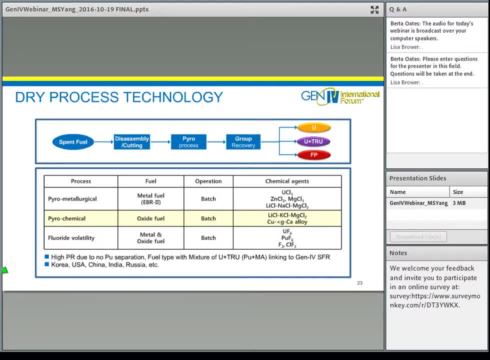 So there are several dry processing technologies. So the pyro-metallurgical process is developed for the metallic fuel fabrication at the EBR2 program in the USA in the early 1950s And the pyrochemical processes are under development in South Korea, USA, China, India, Russia. 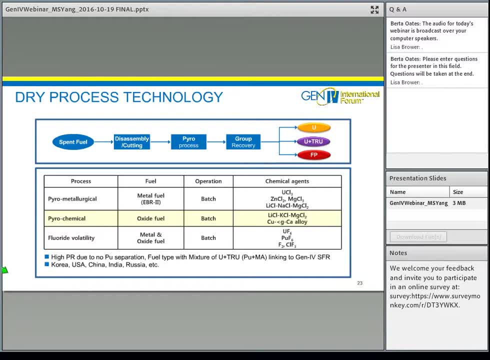 and the fluoride volatility process are mainly for treating the research director fuel. So the dry process has a high proliferation resistance because it does not separate pure plutonium And the fuel with the mixture of uranium, plutonium and the minor actinide can be fabricated. 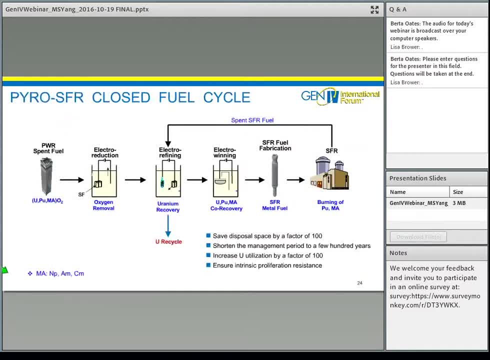 and to be used at the Gen 4 type reactor. So this is the dry process, And the fluoride volatility process is mainly for treating the research director fuel. So the dry process has high proliferation resistance because it does not separate pure plutonium. plutonium and the minor actinide can be fabricated and to be used at the Gen 4 type. 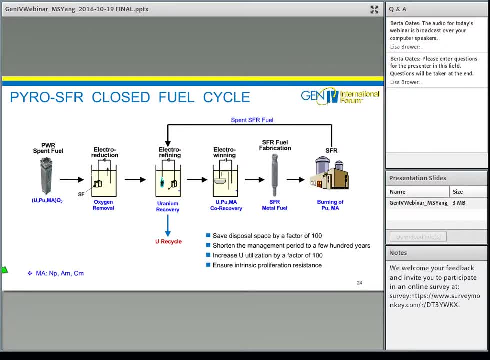 reactor And the fluoride volatility process is mainly for treating the research director fuel. So this slide shows the closed fuel cycle for the pyro processing linked with the sodium fast reactor. So at first the PWL spent fuel is disassembled, Then the spent fuel material is located, will be located at the cathode basket and the 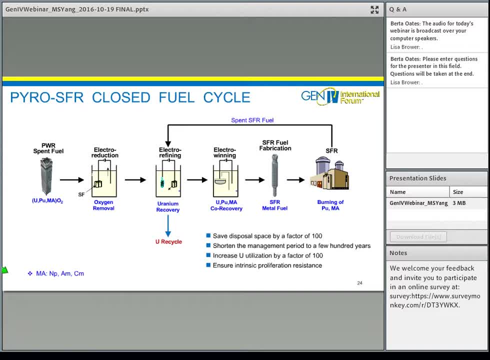 anode is made of platinum, Then electrolytic reduction will take place in the molten salt, and the uranium and the TiO2 will be reduced to the metallic form. here The next stage is the electro-defining process, Here the metallized uranium. 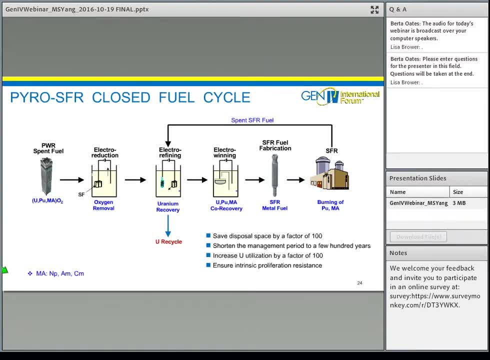 plutonium and the minor actinides and the fission products are placed as anode, and here uranium will be recovered as a solid cathode and the TiO2 and the fission products and the residual uranium will be dissolved in the soil and the next process is the electro-renewing process. So by using 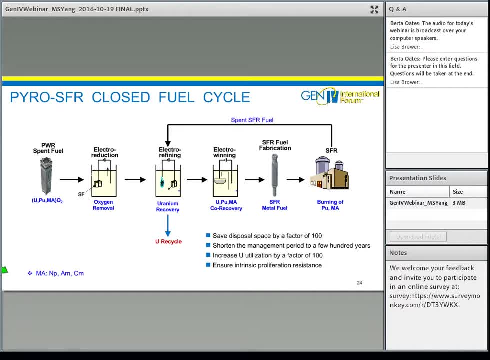 heated cadmium as a cathode. uranium and TiO2 material in the soil can be recovered as the cathode. then cadmium will be distillated. then recovered uranium and the TiO2 material can be used for the sodium phosphoryl. 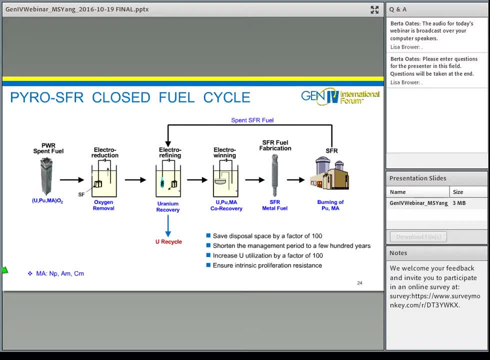 copper fabrication. So by using the sphincter in this way, the uranium utilization can be increased by a factor of 100 and also the volume of the high-level waste can be reduced. And moreover, as the sodium phosphorylated can burn, the long-lived. 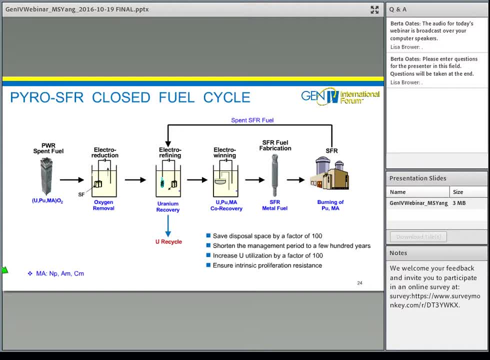 taxi values. it can reduce radio-toxicity, decreasing time, and this means you can shorten the management period of the deep geological repository to a few hundred years. In this pyro processing, there are no streams of pure plutonium separations, and the product is a mixture of uranium and tiallium materials. So this process can delay the during мои 지금은 통제 국. apologise amid 임 battery overheating. this process can delay the joining of uranium and tiallium produto proceed тест and speed up 20 ohm per meter surface. למ� quería real 송 được. So near the bottom half of the of uranium and tiallium muta, Addflux 오 Parliament in order to ensure that the side long and more systemic首先. but it shouldn't beそう 그外 이상 재�状성으로 혜효가你想 Tam powers to be likely if there is more water present than chemical fields. 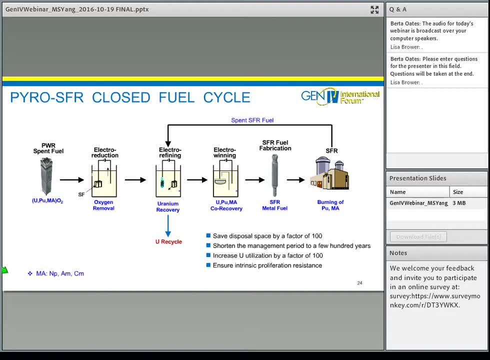 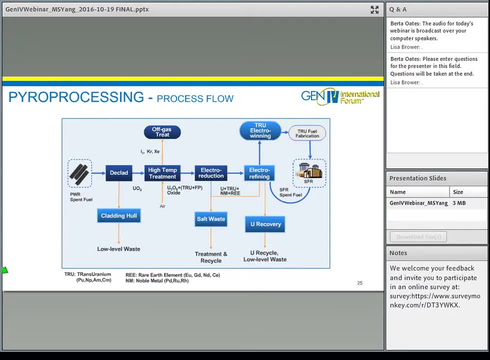 can be considered as a highly proliferation resistant. This slide shows the material flow in the pyroprocessing. So the spent fuel is disassembled and the lot elements are cut to small pieces. Then the lot cuts are declared by mechanical and thermal methods. 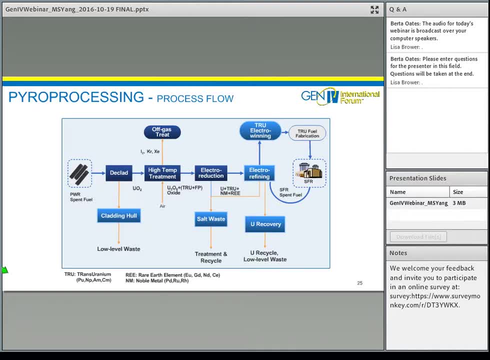 And then we cover the fuel materials subject to the high-temperature treatment to get rid of off-gas like iodine, krypton and xenon. Then the oxide material composed of uranium, TRU and fission products are reduced to the metallic form. 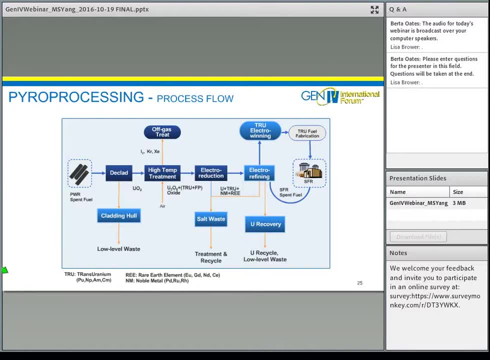 at the electro-reduction process. Then the metallic uranium, TRU, noble metal and rare earth elements are treated by the electro-reduction to recover uranium And then treated by the uranium refining to recover the uranium and treated by the electro-reducing to recover. 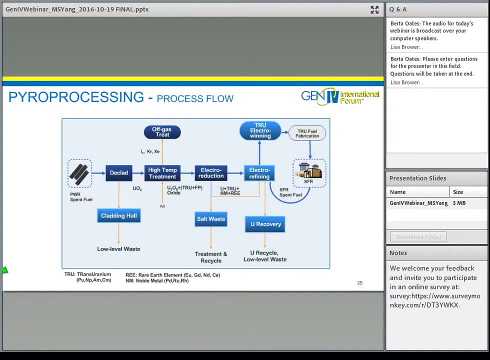 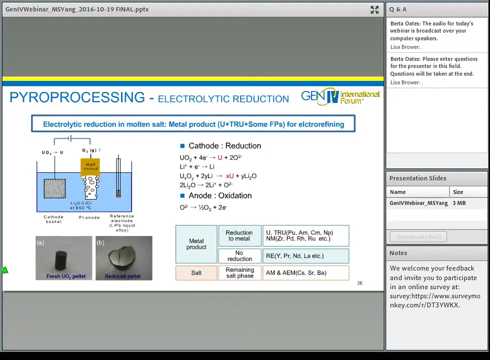 the material, And then the uranium and material will be used for the sodium fossil fuel fabrication, And then the spent SFR fuel will again be recycled. in this way to close the system. Thank you, Thank you, Thank you, All right. well, that's all the information. 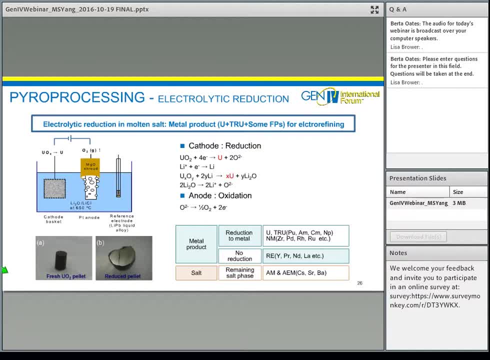 about and the noble metal like zirconium and palladium will be reduced to a metallic form, but rare earth elements like yttrium are not reduced and the alkali material and alkali earth material like cesium and strontium will be remained in the soil. 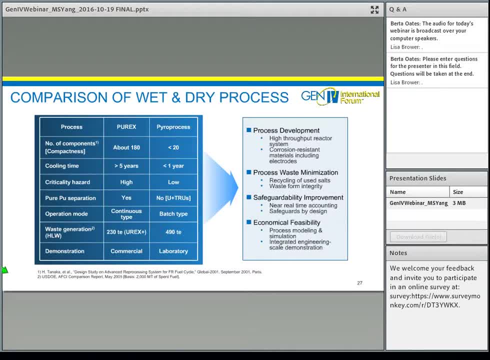 So this is a conceptual comparison of this wet and dry recycling route. So, regarding the complexity of process, that means the compactness of the process. pyro processing is rather compact And for the cooling time needed for the spent fuel to be processed, purex process requires. 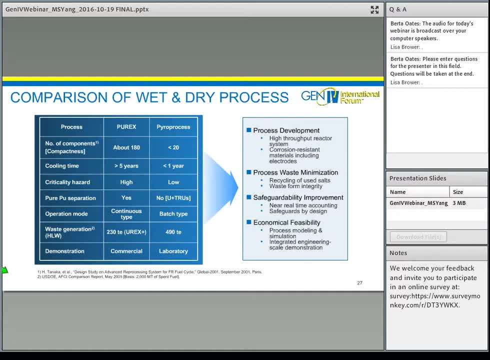 more than five years cooling to be treated, But pyro processing can process spent fuel that is just cooled about one year. And regarding the criticality hazard, the purex process has a high criticality because you use the wet process And the purex process can separate the pure plutonium. but in case of pyro processing, 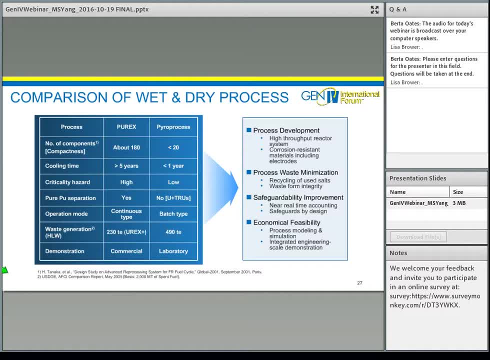 the pure separation of pure plutonium is not possible And the pyro processing is just under development in the laboratory scale and while the purex is already commercialized in the world. And, moreover, the pyro processing is producing more process waste and it is basically a batch. 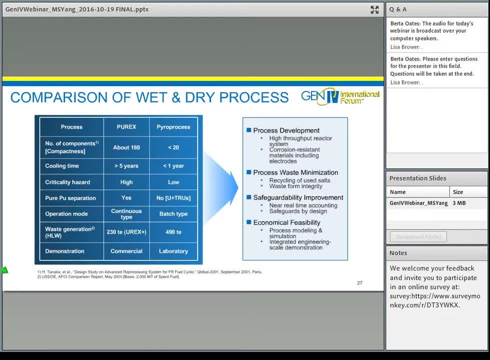 type process. So you need more development for the large scale production. So can you see the difference? Yes, So currently there are R&D efforts to improve the pyro processing. The research objectives are for the process development. it is to develop high throughput. 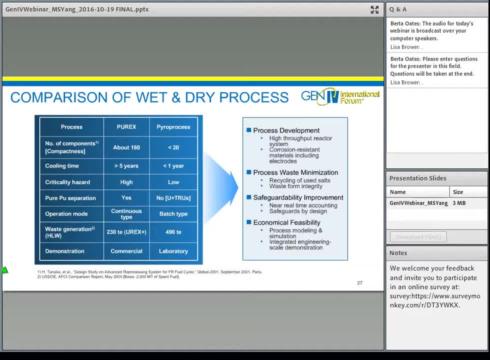 process and to develop corrosion resistant material. And the second is for the process: waste minimization by recycling the used salt. And the third is to improve the pyro processing. And the fourth is to improve the safeguard ability by developing near real-time accounting techniques. and design improvement of the facility design stages. 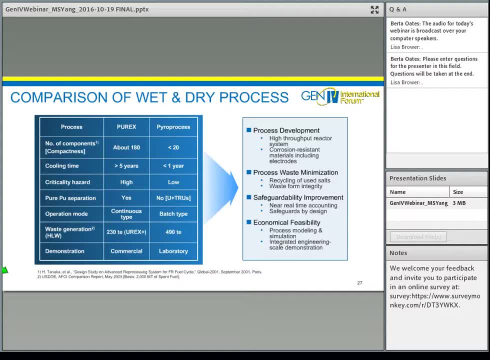 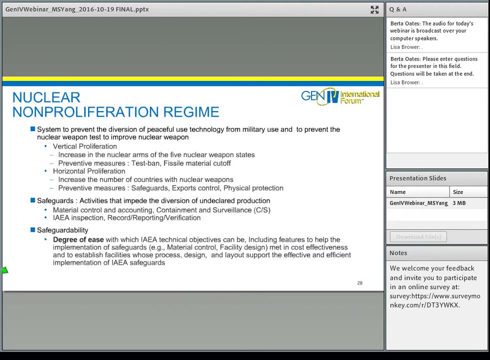 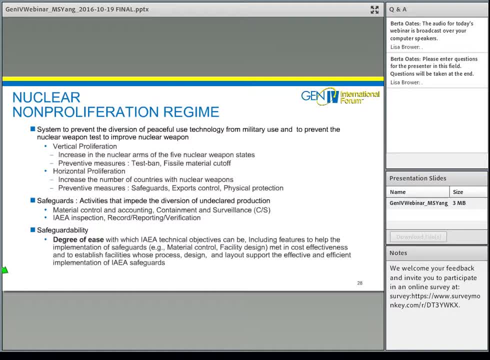 Thank you. So when we are dealing with nuclear fuel cycles, one important issue is nuclear non-proliferation. So from the beginning of IAEA, the international effort were made to encourage peaceful use of nuclear energy while ensuring prevention or diversion of nuclear technology. 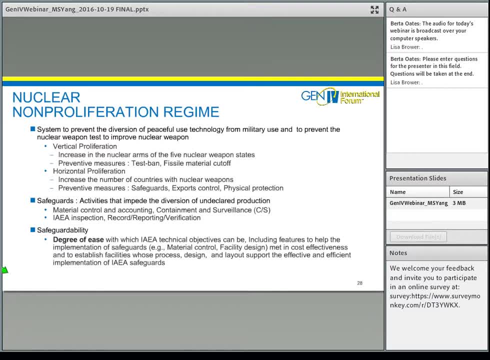 So nuclear nonproliferation regime means that the cost of nuclear energy will be reduced all over the world. So, as we discussed earlier the— settings that I alluded to are in the top left. government purposes regime means the system to prevent the diversion of peaceful use technology to a military use. 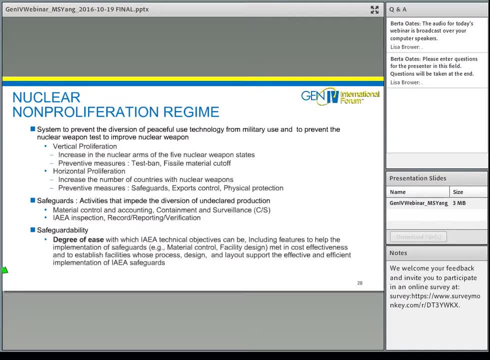 and to prevent the nuclear weapon test to improve it. So the latter is called vertical proliferation and the former is called horizontal proliferation. Vertical proliferation means increasing the number of countries with nuclear weapons. So for the prevention of the horizontal proliferation there are various preventive measures, like 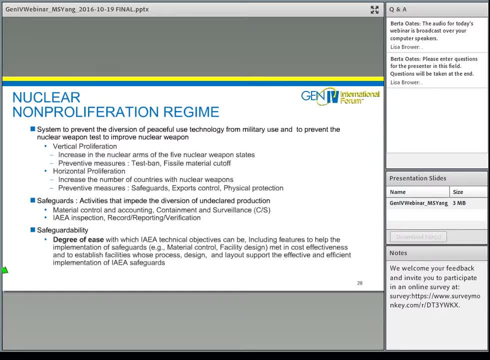 safeguards and export control and the physical protection, And among them safeguards measures, play the most important role. So the safeguards can be used in many ways. So the safeguards can be used in many ways. The first one can be defined as the old activity that impedes the diversion of undeclared production. 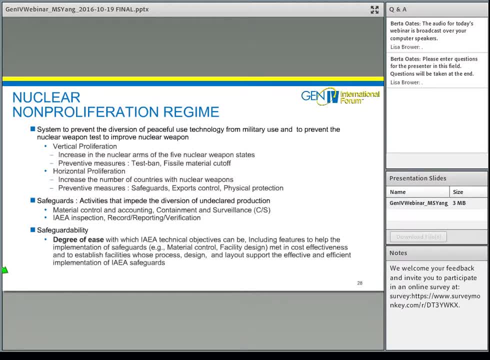 of nuclear materials, So it's composed of material control and accounting, and containment and surveillance. And IAEA inspection, including the recording, reporting and verification, is also important activities And, moreover, when we develop new fuel cycle technology, we had better consider the safeguard. 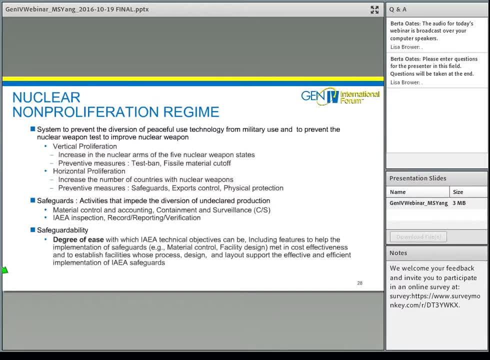 ability of the process in advance to make the process easy to be safeguarded. The safeguard ability is defined as the degree of easy with which IAEA technical objective can be met. The second one can be defined as the cost effectiveness of the process while maintaining 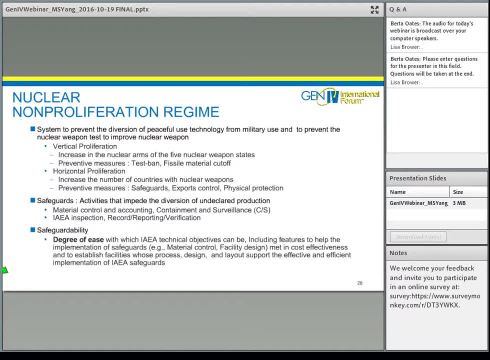 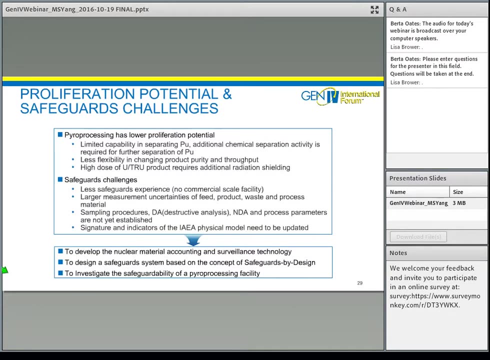 the cost efficiency and the availability of the first stage of the process. In addition, the most important function of the process is the best tool for the related mechanics and the cost effectiveness and to establish facility whose process design layouts support the effective and efficient implementation of IAEA safeguards. 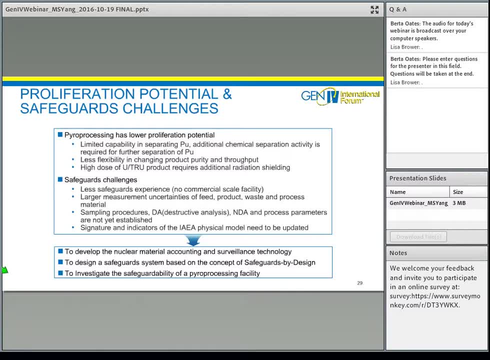 So the pilot process has a better or lower proliferation potential compared to with other fuel cycle technology, because in the next phase the pipeline will be also much more effective. it has a limited capability in separating pure plutonium and also it has less flexibility in changing the product purity and throughput. and the high dose of uranium and the trial. 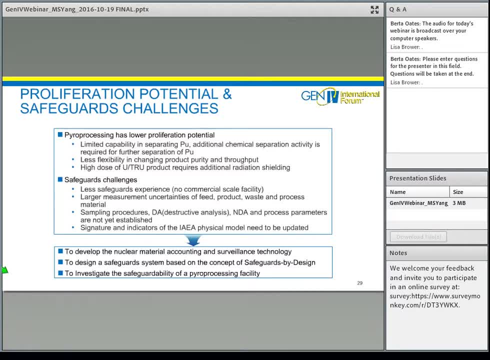 product requires additional radiation shielding, so it makes the diversion very difficult. however, it needs more development to solve safeguard challenges for the pyro processing. so the first is there are less experience for the safeguard practice because there are no commercial scale pyro processing facility yet, and secondly is there are larger measurement uncertainty of 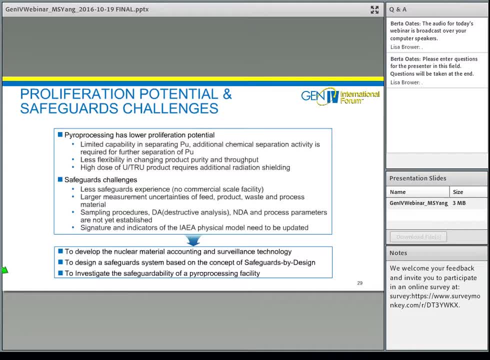 feed product weight and efficiency. and third is sampling procedures, including destructive analysis and non-destructive analysis, and the process parameters are not well established yet and, moreover, a current signature and the indicator of IAEA physical models needed to be updated for the pyro processing application. 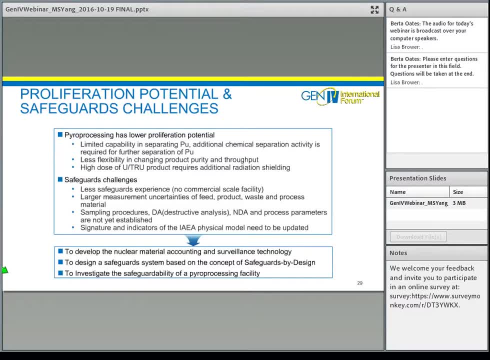 so therefore, in parallel to the process technology development, the safeguard R&D has better be performed simultaneously. so the R&D area for the safeguard of the pyro processing are to develop the nuclear material accounting and surveillance technology and to design the safeguard system based on the concept, so-called safe guard system based on the concept, so-called 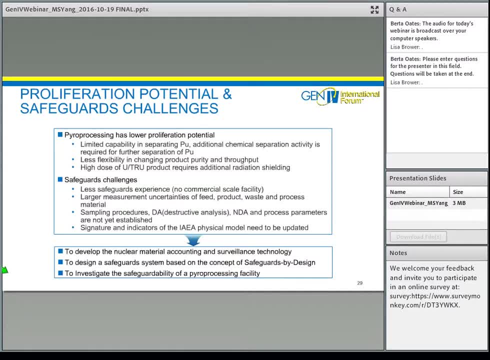 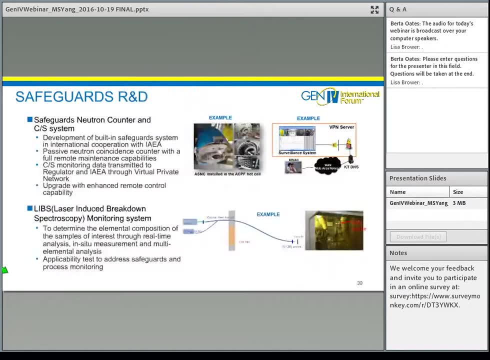 safeguard by design and to investigate the safeguard ability of pyro processing facility, and this slide shows some examples of safeguard R&D. so safeguard neutron counter is to measure the amount of sensitive material in non-destructive methods and this is a passive neutron coincidence counter is a full remote maintenance capability. 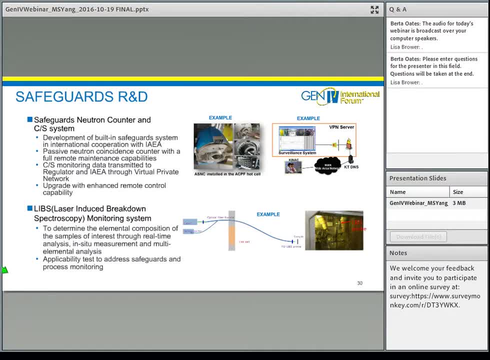 And another one is containment and surveillance system development. This containment and surveillance monitoring data is transmitted to the regulatory body and the IAEA through virtual private network. And another example is to develop laser-induced breakdown spectroscopy monitoring system. So this is to determine the elemental composition of the samples through real-time analysis. 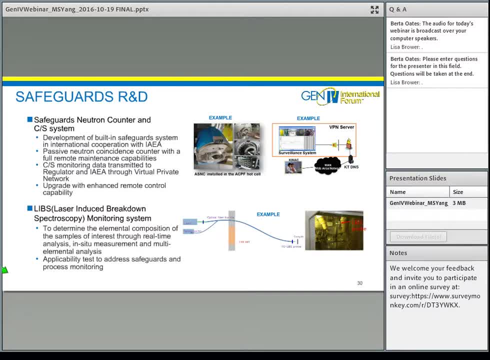 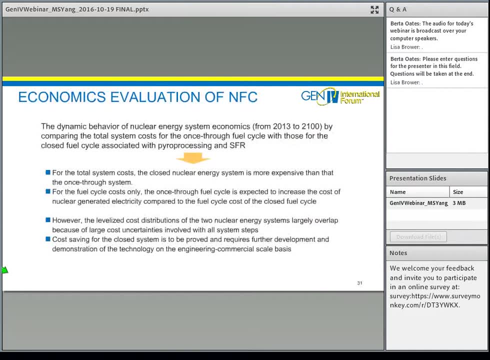 And by using this system, the in-situ measurement and the multi-element analysis will be possible. And before making a decision, I would like to make a comment. Before making a decision to invest in a big project, we need to perform the economical. 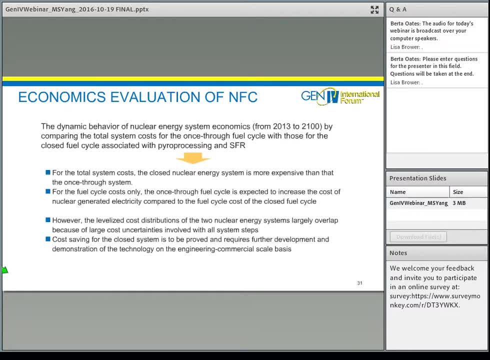 analysis of the fuel cycle, So the dynamic behavior of the nuclear energy system, nuclear energy system economics, was performed by comparing the total system cost for the one fuel cycle with those for the closed fuel cycle associated with the pyro processing and SFI. So the tentative study results shows that, for example, regarding the total system cost, 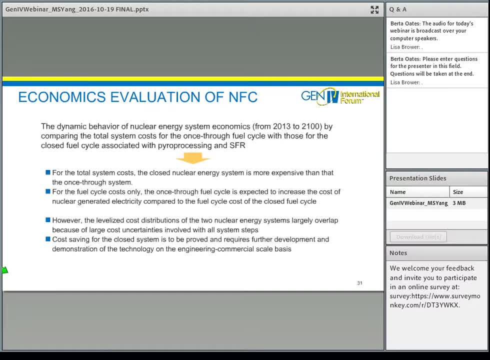 the closed nuclear energy system is a little bit more expensive than that of one-through system, But regarding the fuel cycle cost, only the one-through fuel cycle is expected to increase the cost of electricity By about 7% compared to that of the closed fuel cycle. 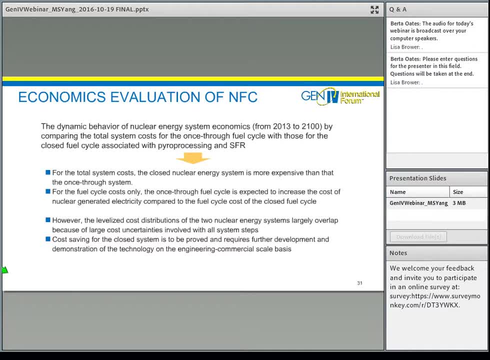 However, the levelized cost distribution of the two nuclear systems is very similar because of large cost uncertainty involved with all the system steps. So it requires further technology development And the demonstration on the engineering commercial scale basis in order to prove the cost saving for the closed system. 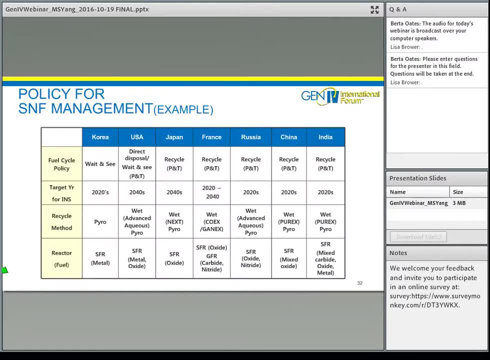 And this slide shows some representative comparison of nuclear fuel cycle policy of the major countries in the world. For example, in Korea the fuel cycle policy will be determined later, The so-called nuclear fuel cycle policy. And this slide shows some representative comparison of the nuclear fuel cycle policy of the major 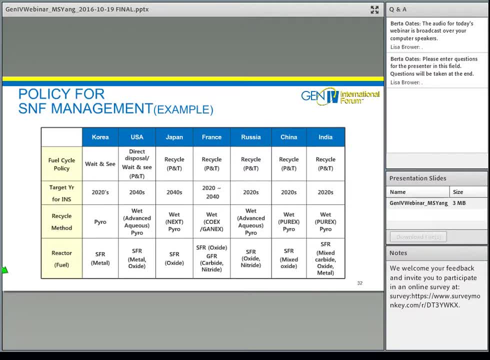 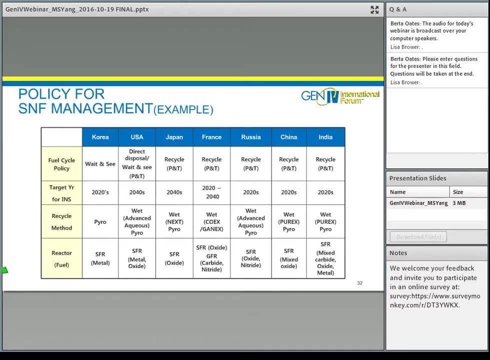 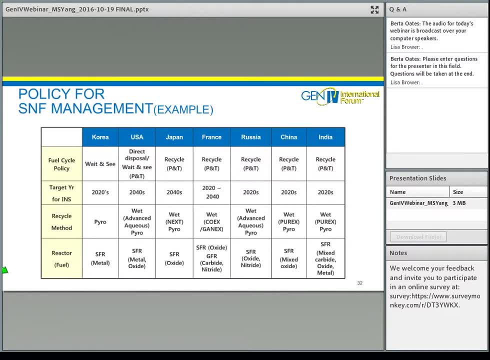 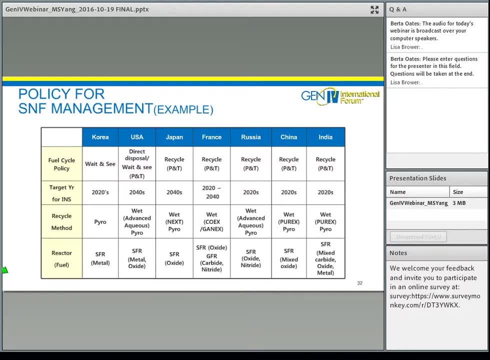 in the world. And this slide shows some representative comparison of the nuclear fuel cycle policy of the major countries in the world. And this slide shows some representative comparison of the nuclear fuel cycle policy of the major countries in the world. And this slide shows some representative comparison of the nuclear fuel cycle policy of the major 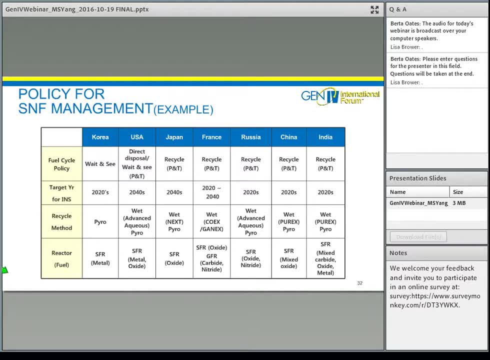 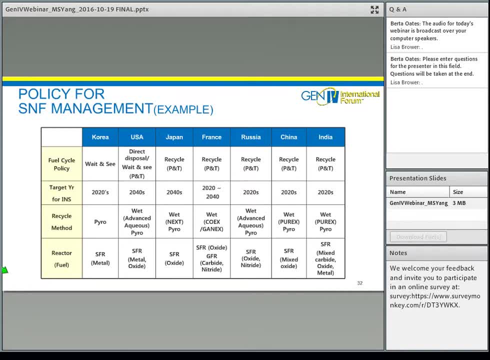 countries in the world. And this slide shows some representative comparison of the nuclear fuel cycle policy of the major countries in the world. And this slide shows some representative comparison of the nuclear fuel cycle policy of the major countries in the world. And this slide shows some representative comparison of the nuclear fuel cycle policy. 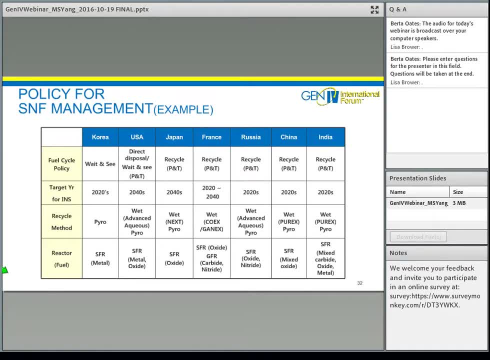 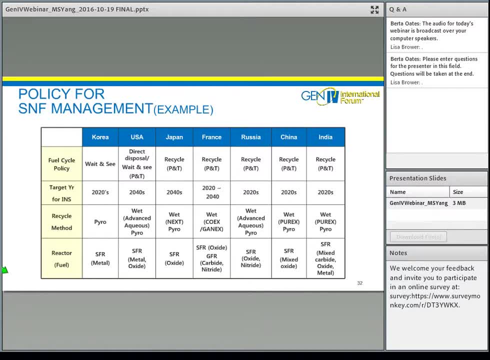 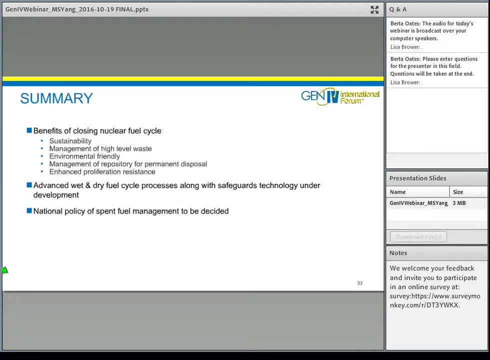 countries in the world. And this slide shows some representative comparison of the nuclear fuel cycle policy of the major countries in the world. And this slide shows some representative comparison of the nuclear fuel cycle policy of the major countries in the world. And this slide shows some representative comparison of the nuclear fuel cycle policy. 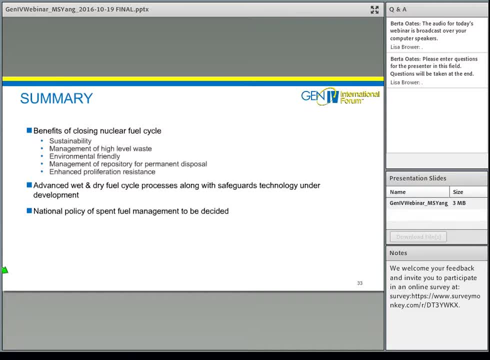 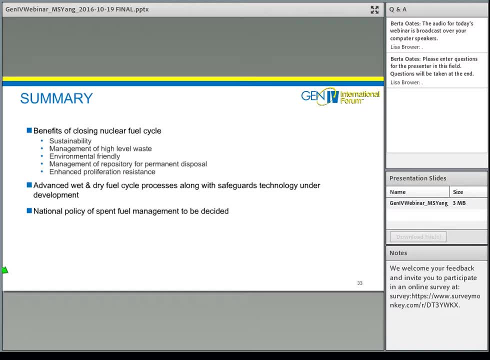 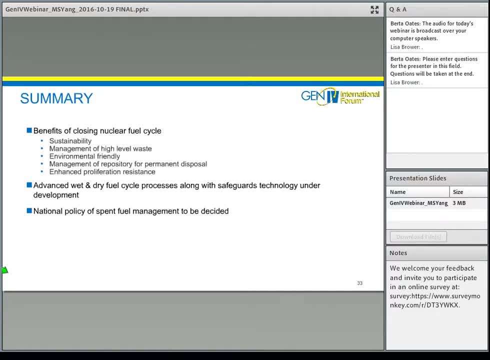 countries in the world. And this slide shows some representative comparison of the nuclear fuel cycle policy of the major countries in the world. And this slide shows some representative comparison of the nuclear fuel cycle policy of the major countries in the world. And this slide shows some representative comparison of the nuclear fuel cycle policy. 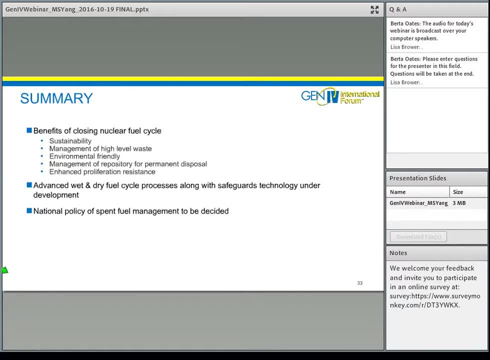 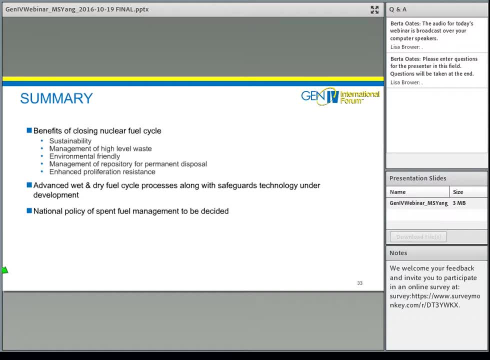 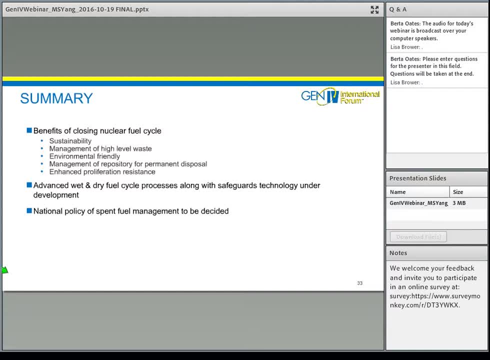 countries in the world. And this slide shows some representative comparison of the nuclear fuel cycle policy of the major countries in the world. And this slide shows some representative comparison of the nuclear fuel cycle policy of the major countries in the world. And this slide shows some representative comparison of the nuclear fuel cycle policy. 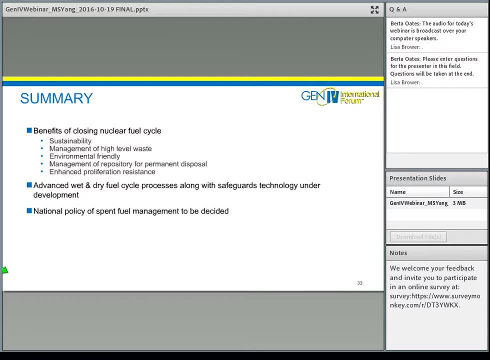 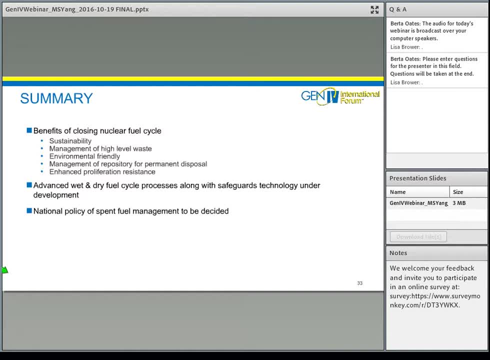 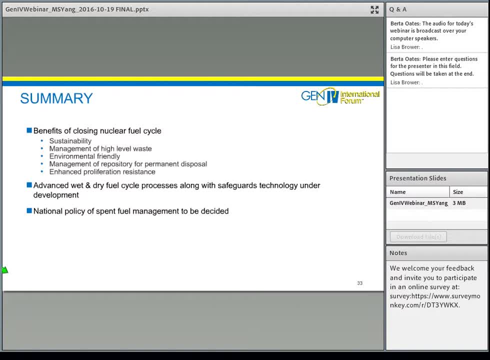 countries in the world. And this slide shows some representative comparison of the nuclear fuel cycle policy of the major countries in the world. And this slide shows some representative comparison of the nuclear fuel cycle policy of the major countries in the world. And this slide shows some representative comparison of the nuclear fuel cycle policy. 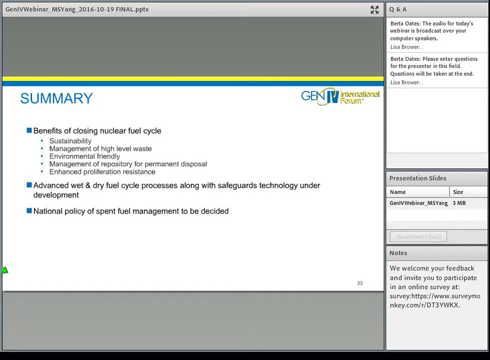 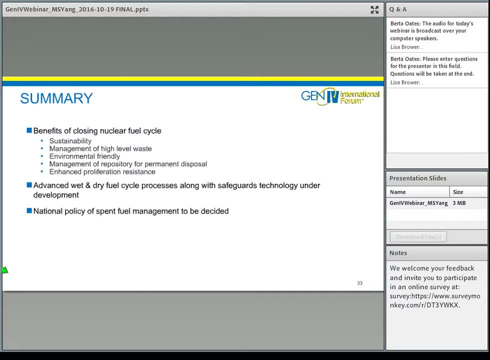 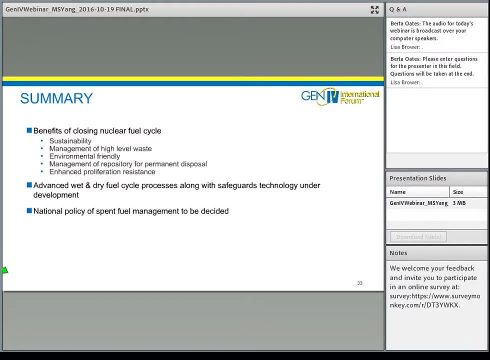 countries in the world. And this slide shows some representative comparison of the nuclear fuel cycle policy of the major countries in the world. And this slide shows some representative comparison of the nuclear fuel cycle policy of the major countries in the world. And this slide shows some representative comparison of the nuclear fuel cycle policy. 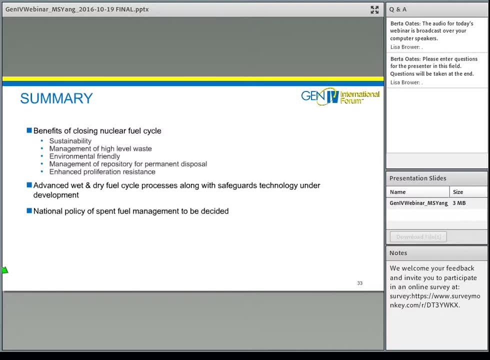 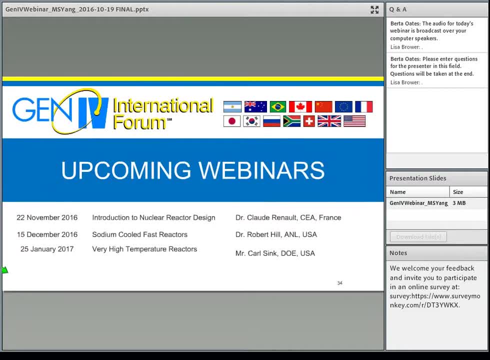 countries in the world. And this slide shows some representative comparison of the nuclear fuel cycle policy of the major countries in the world. And this slide shows some representative comparison of the nuclear fuel cycle policy of the major countries in the world. And this slide shows some representative comparison of the nuclear fuel cycle policy. 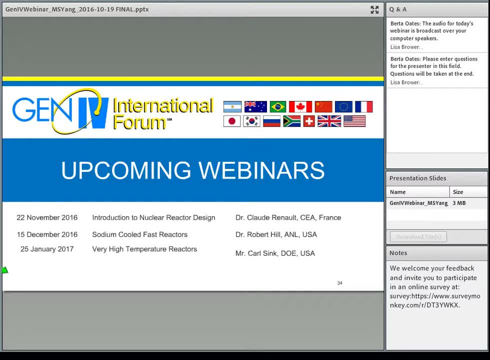 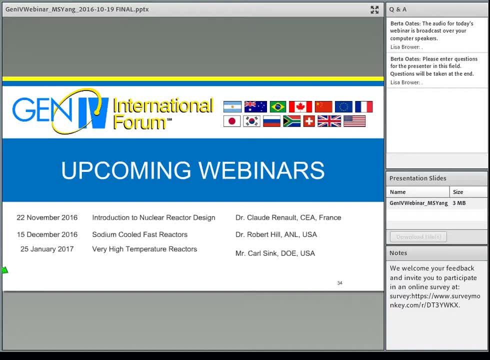 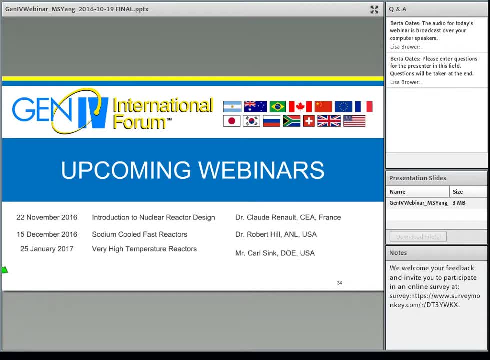 countries in the world. And this slide shows some representative comparison of the nuclear fuel cycle policy of the major countries in the world. And this slide shows some representative comparison of the nuclear fuel cycle policy of the major countries in the world. And this slide shows some representative comparison of the nuclear fuel cycle policy. 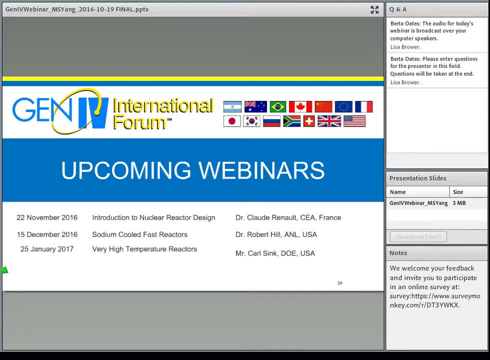 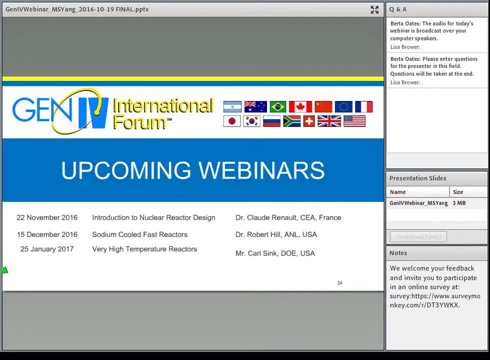 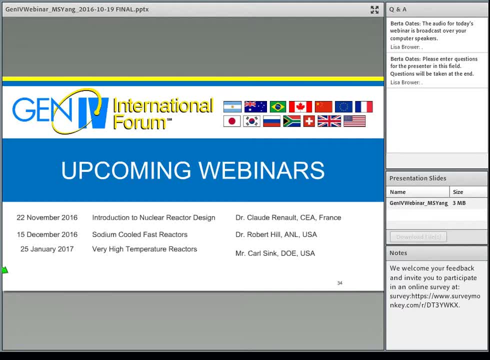 countries in the world. And this slide shows some representative comparison of the nuclear fuel cycle policy of the major countries in the world. And this slide shows some representative comparison of the nuclear fuel cycle policy of the major countries in the world. And this slide shows some representative comparison of the nuclear fuel cycle policy. 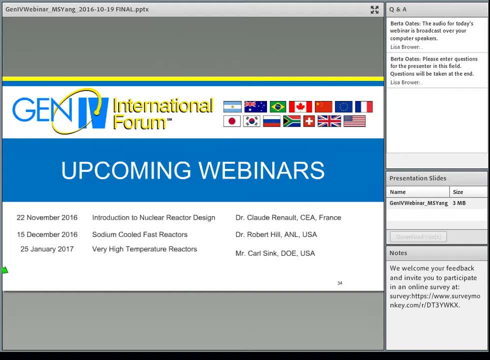 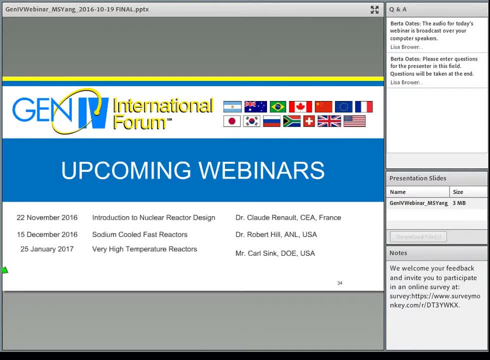 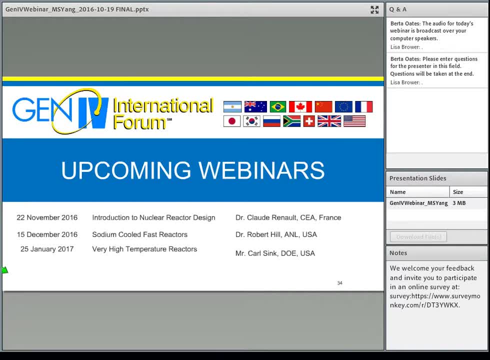 countries in the world And this slide shows some representative comparison of the nuclear fuel cycle policy of the major. The first question is: are there currently any plans to use most fuel in commercial USA in the USA? So I think we had a better answer to that question. 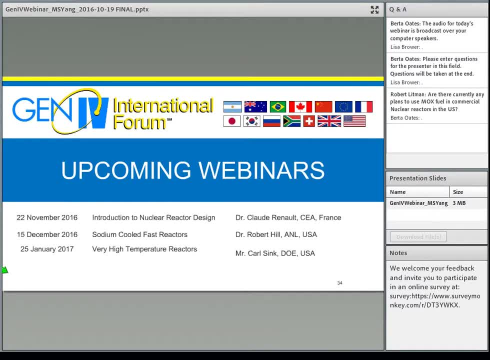 I'm sorry, Oh, Patricia. So the first question is from Dr Littleman, but I think that question is: are there any currently plans to use most fuel in the USA? So I think you had a better answer to that question for me. 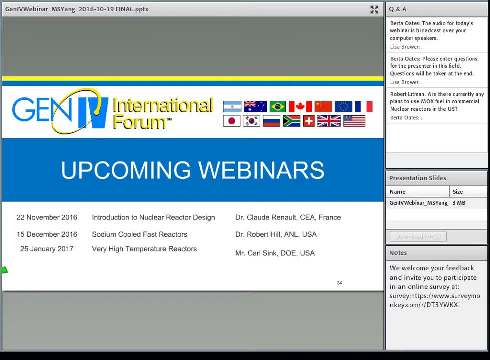 Yeah, Okay, So this is Patricia Pavia from DOE, and no, for the moment there's no plan to use mixed oxide fuel In the US. Dr Littleman also has a question about cesium-137,, strontium-90, and emery-341. 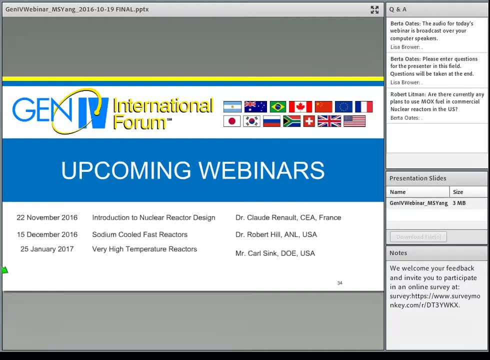 Yes, I think also. the question is that had better be answered by Patricia, right? Okay, And I don't see the question better. Okay, I see it now. So the question is: are there any plans to use most cesium-137,, strontium-90, and emery-341? 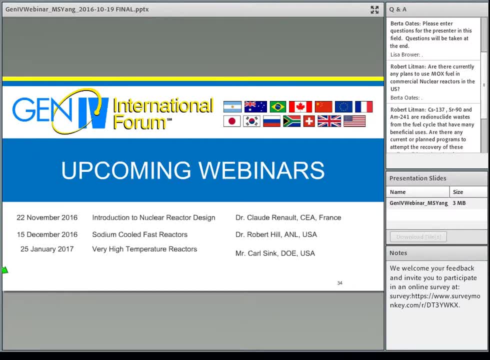 from the fuel cycle that have many beneficial uses. Are there any current or planned programs to attend the recovery? Okay, In the United States until 2008,, we developed the UX process, where there was a plan to extract cesium and strontium. 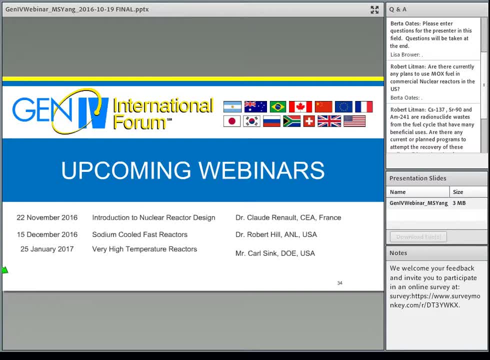 But unfortunately, when you go from R&D to engineering scale and then industrial scale, there was no plan to use cesium-137,, strontium-90, and emery-341.. Okay, So the question is, are there any plans to use most fuel in the USA? 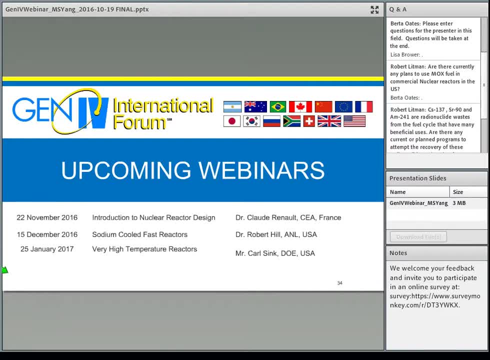 So this is a good question. It's not necessarily equated to the fact that we have the energy we need, but I think that's the first step. So I don't think that the UX process is the best. I do think it's possible. 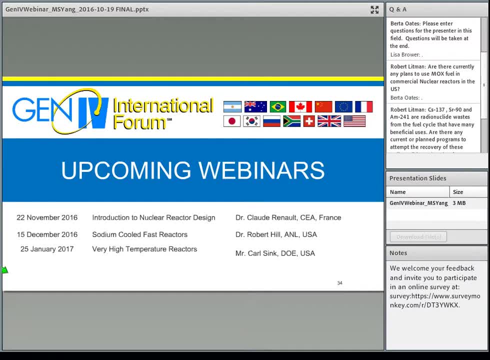 Right, the spent fuel in nitric acid. and then we have two paths: either a heterogeneous recycling or an homogeneous recycling. homogeneous, we will try to extract all of the actinide of importance, basically uranium, plutonium, neptunium, americium. and for the heterogeneous, we will start with a. 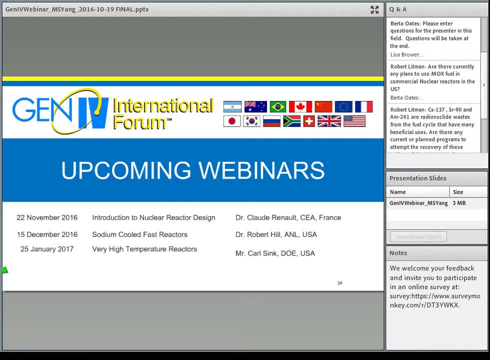 modified PUREX process- uranium, plutonium, neptunium- followed by the ALCEP process, which stands for actinide lanthanide separation process, where you would separate the trivalent actinide americium corium from the trivalent lanthanide. it's using a acidic extract and combined with 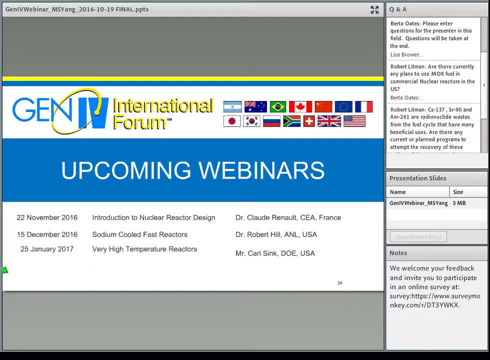 the neutral extractance. so yes, for the americium, we have a lot of research going on. we are also investigating the oxidation of americium 3 to americium 6. thank you. okay, so thank you for you. yeah, so, and the other question is also regarding the thorium fuel. you 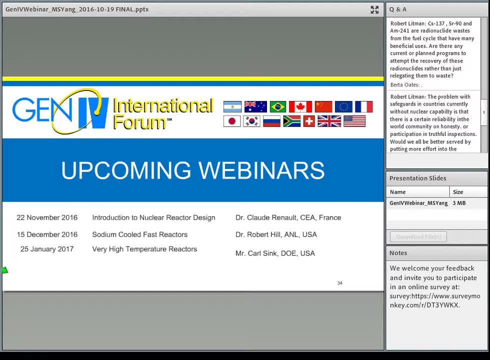 know molten salt and also I think I need some advice from the Patricia. oh, okay, let's see what. um, I do not see the question right now. so a problem with safeguards in countries currently without nuclear capability is that there is a certain reliability in the work community on honesty or participation in through full expansion. would we all be better? 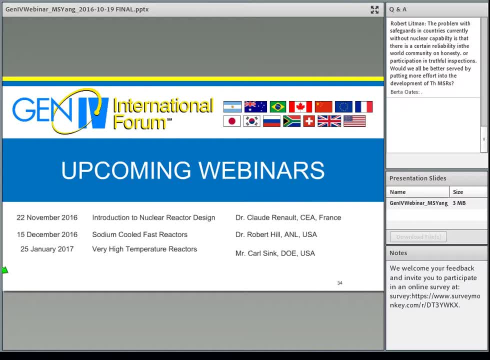 served by putting more effort in the and I don't see the end in the what into the development of thorium MSRs. okay, for the moment the United States are not focusing on the thorium fuel cycle at all. we are focusing on uranium fuel cycle and also the question from the Mr Farah is for the radio toxicity with the spent nuclear fuel treatment. 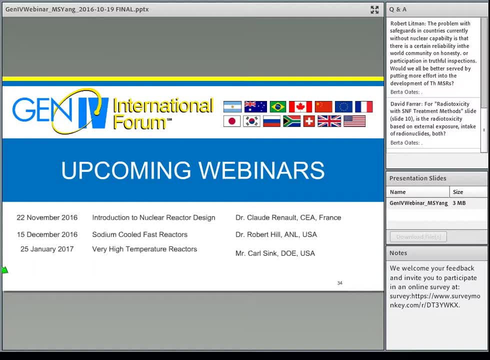 yeah, so actually you are right so that the radio toxicity is based on the external exposure and the intake of the radionuclides together. so you know for the details. so I do not have that material right now, but the radio toxicity is a kind of collective concept. 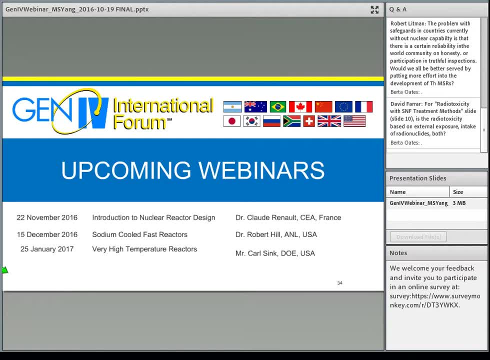 of the nuclear fuel cycle. so the other question is: uh, is there a minimum of nuclear power plant or annual spent nuclear fuel generation for establishing the closing the fuel cycle? yeah, surely? yeah, that is a very good question. and when we perform the economic analysis of the fuel cycle, you know we have to assume the some 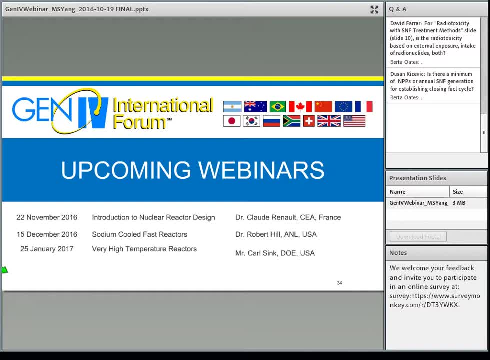 you know, we have to assume the some, the minimum amount of spent fuel, And also that is depending on what kind of nuclear fuel technology we are going to use. So in case of pyro processing, since that is mainly based on the batch type process, so small amounts of spent nuclear fuel can be treated In case of wet process, since that is a continuous process, so they need a large amount of spent fuel. So surely there is some minimum of nuclear power plants and spent fuel generation for closing the fuel cycle. 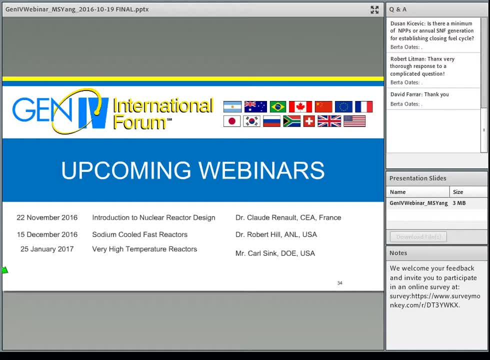 But surely that minimum amount is depending on what kind of fuel cycle technology we are going to use. So the other question is: what are the issues that need to be resolved before power plants and pyro processing become commercialized? That is also a very challenging question. 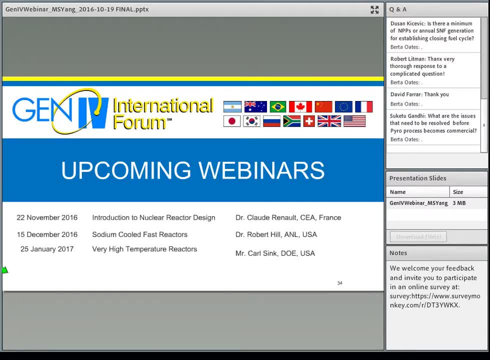 Nowadays, the feasibility of pyro processing is proved just at the laboratory level. So, to become that, in order for that pyro process to become commercialized, surely you have many technology obstacles, Surely, to find the I don't know. 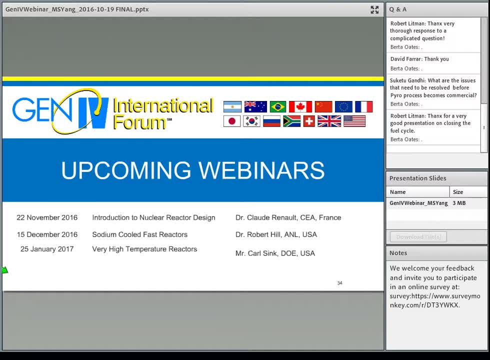 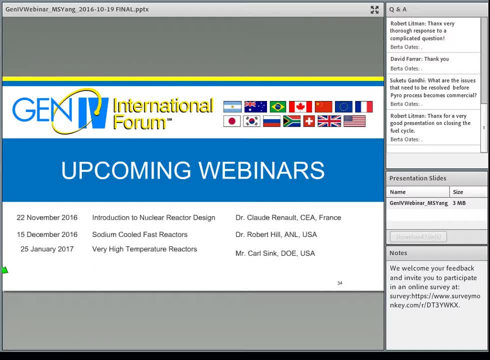 challenge. But the big challenge is mainly pyro processing is the batch type process. So to be commercialized or to have a large scale processing of the pyro technology will be a challenging one. So that is why we are performing that kind of researches. 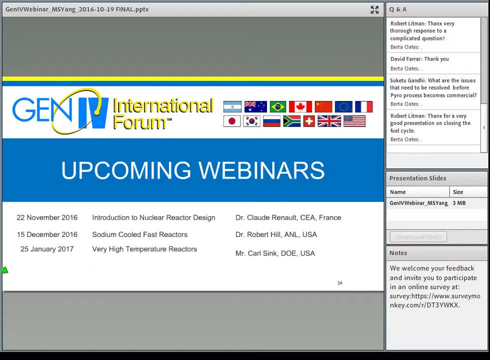 So in coming five years the So feasibility of pyro processing will be evaluated in terms of technical feasibility and the safeguard ability and also in terms of economics. So maybe I can answer more clearly in coming five years later, about five years later. 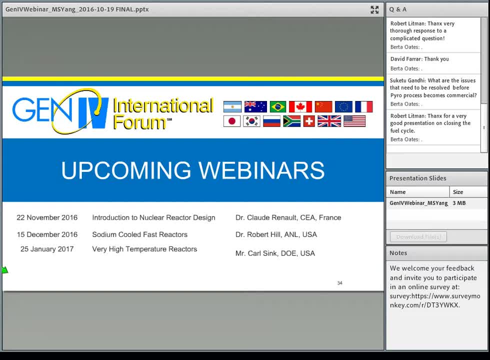 Great. but the next question deals with research by the AEC in the 1960s. Let me see, I know there was research by the AEC in the 1960s into the SFRs in the USA. What is the current direction towards the use of this type in the USA? 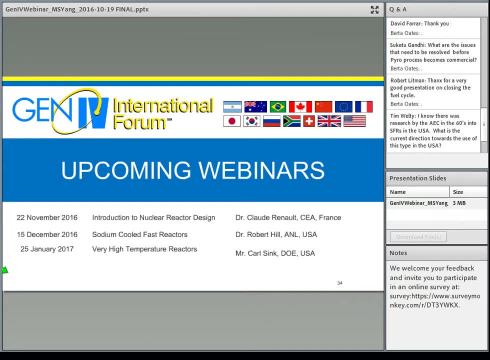 So also, I need, you know, I need advice from Patricia. Yes, Right, We're going to have actually a presentation and I refer Tim Welty who asked: I know there was research by the AEC in the 60s into sodium fast reactors in the USA. 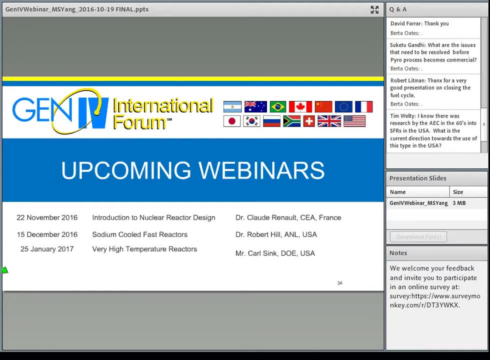 What's the current direction towards the use of this type in the USA? Bob Hill from Argonne National Laboratory is our national technical director and I really invite you to listen to his webinar in two months, on the 15th of March, And I guess he will answer your questions.